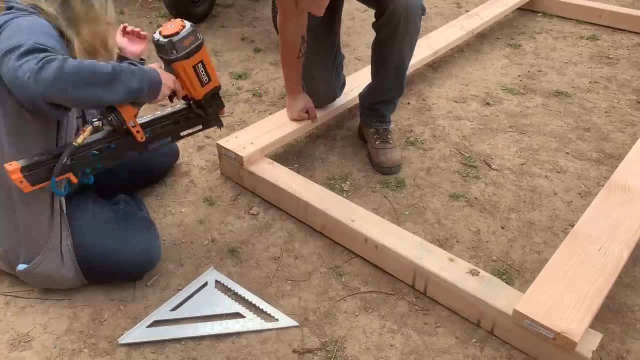 And I'm just going to attach one of the 2x6s here to one of the vertical 4x4s Now for each planter box, the 4x4s that are tall. they're going to be tall on one side. 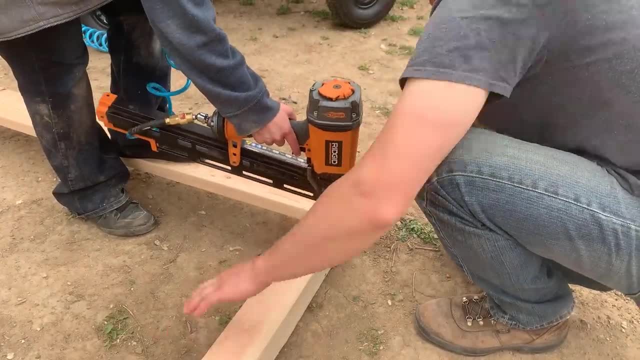 That's going to be the outer perimeter and that's what I'm going to attach the fence to, And then the ones that are on the inner perimeter of the planter box walls are just going to be a lot shorter, And we're just going to make sure that we have enough space. 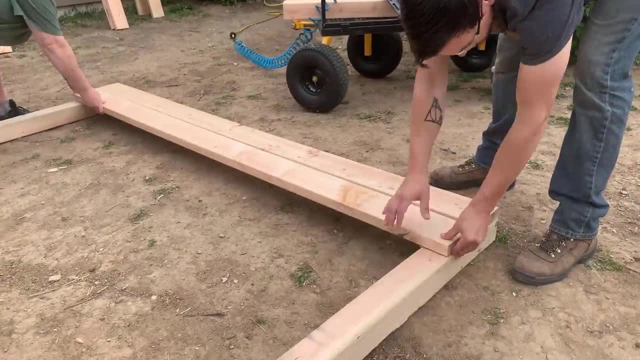 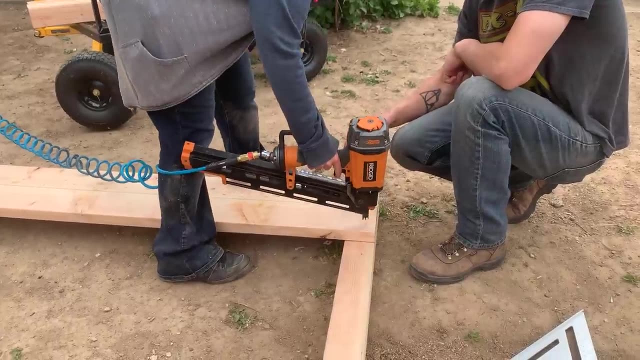 So I'm just going to use nails. I'm actually using a ring-shanked galvanized nail, so the nails aren't going to rust, And you can see my daughter, Maya, is doing the bulk of the assembly here and she's with her boyfriend who's helping us out. put these things together today. 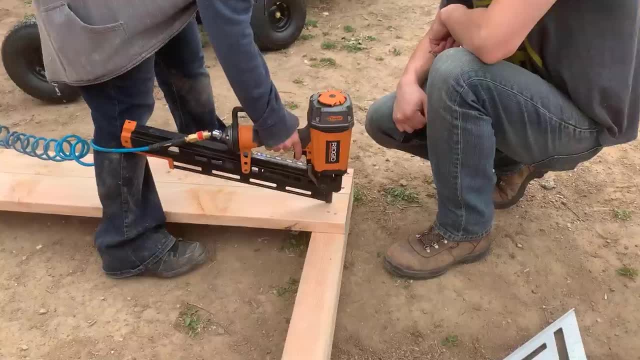 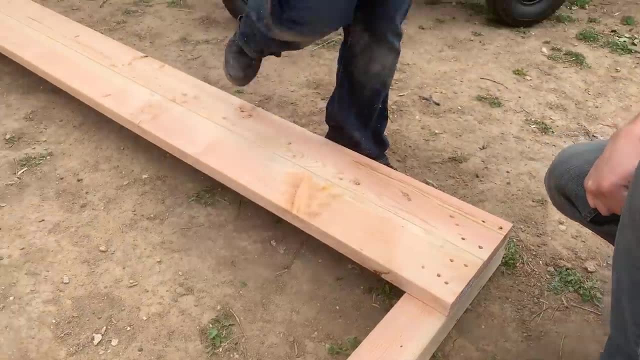 It's actually a pretty simple project too. it's something you can do in one or two days. It doesn't take a whole lot of time to put together something like this. So you're going to be wondering why would I bother to use ring-shanked galvanized nails if I'm just going to use Douglas fir? 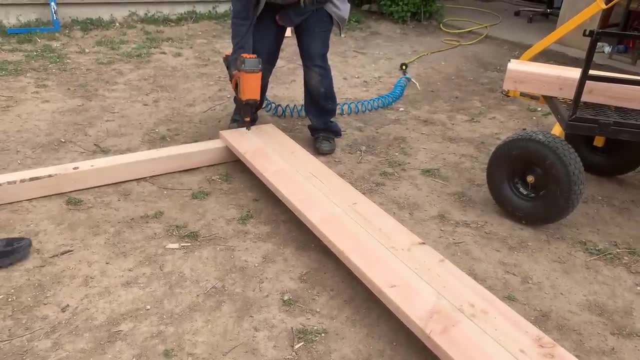 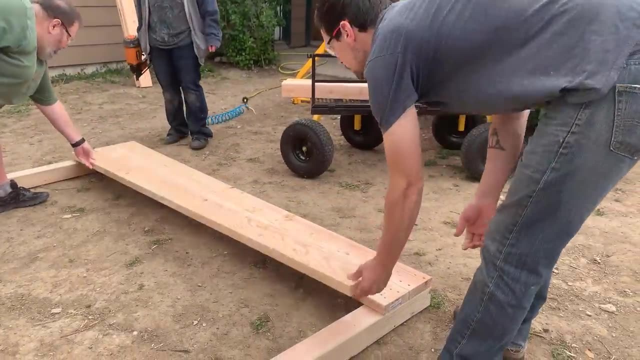 And the reason I'm using Douglas fir is because I built a planter out of it. actually, more than one occasion I have done. I've built a little short planter out of it that I've set on the ground outside And after ten years the planter still was not rotted all the way through. 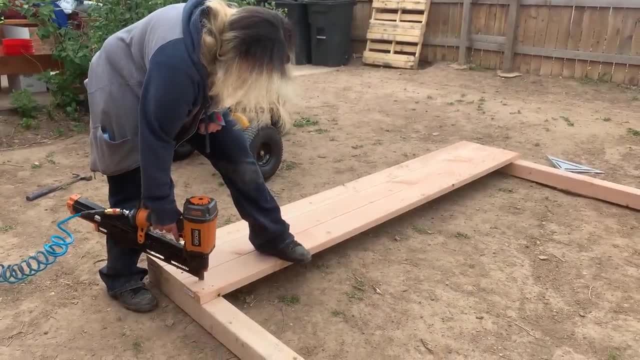 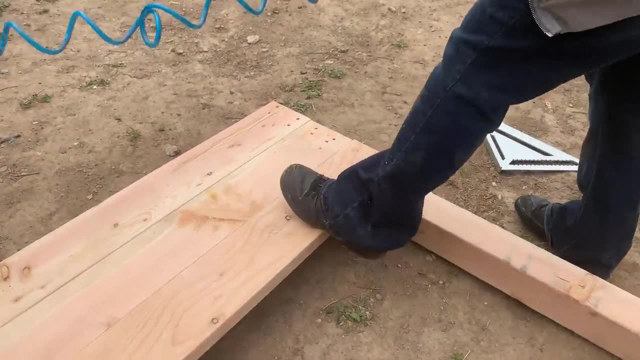 In fact it held the dirt just fine and there was no problem. I've actually also built small planter boxes, little round circular planters and little round square planters that we've set out in the yard, made of Douglas fir, And I've made them out of southern yellow pine that weren't treated. Those have also lasted more than ten years, In fact, by the time they got around to where they would have probably rotted anyway. I was tired of them and we wanted to get rid of them, And I don't know that I want to have this garden in the backyard for the rest of my life. 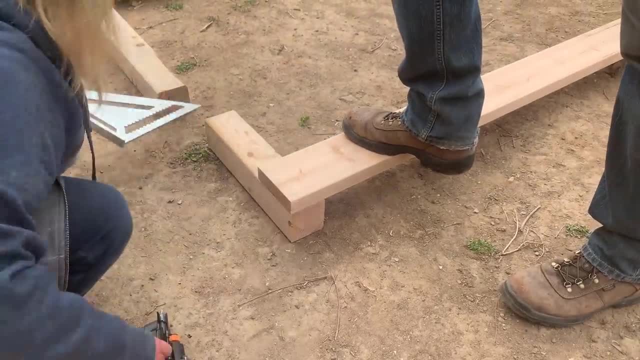 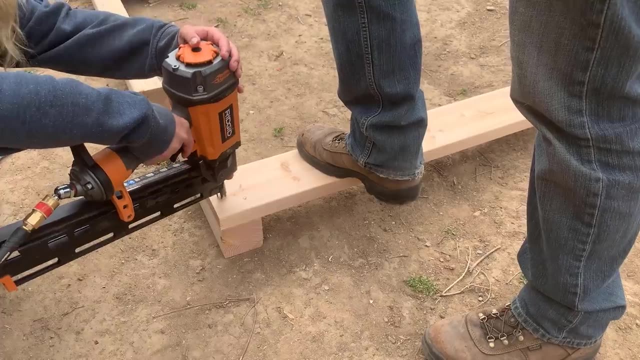 So rather than spend twice the money on cedar or one and a half times the money on some sort of a pressure treated which I'm not comfortable with, the chemicals in that I figured it would be better for me to go ahead and do this out of Douglas fir. 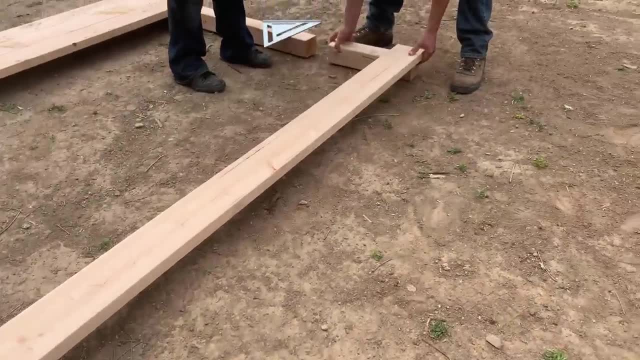 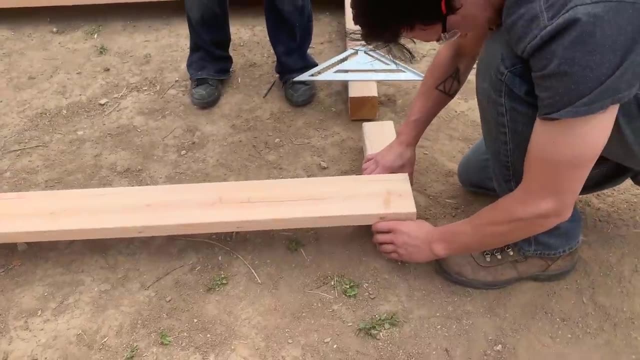 And I know it's going to sit here for at least a decade. Maybe it would sit here longer than that, But I don't know if I'm going to keep it that long anyway, And at any rate it's going to be a good experiment to kind of see what happens as time goes by. 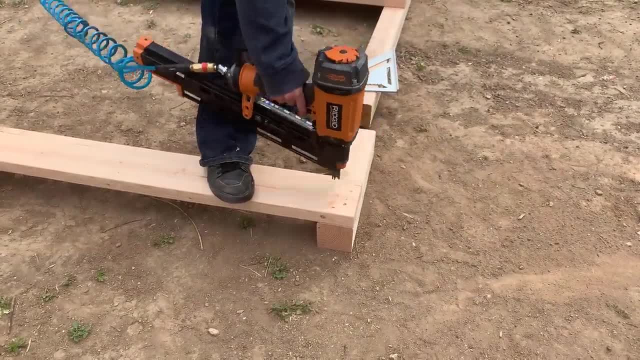 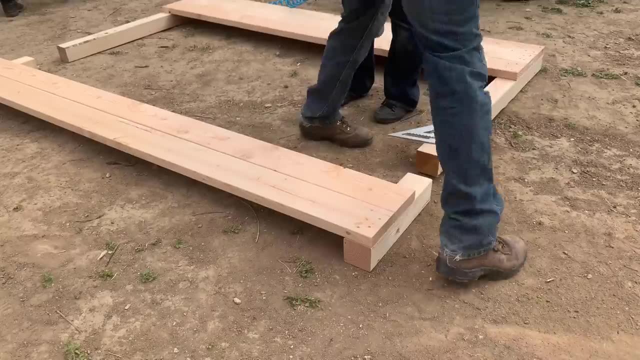 Now, here you can see, Maya is nailing together the short planter wall which will be the side of the planter wall that comes on the inside of the garden, And we've chosen to have three, two by sixes tall, the walls for this planter garden all the way around. 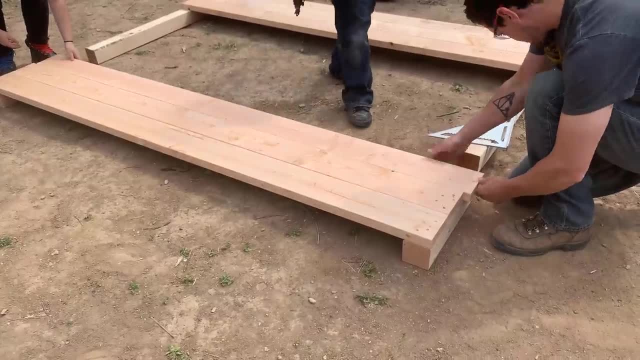 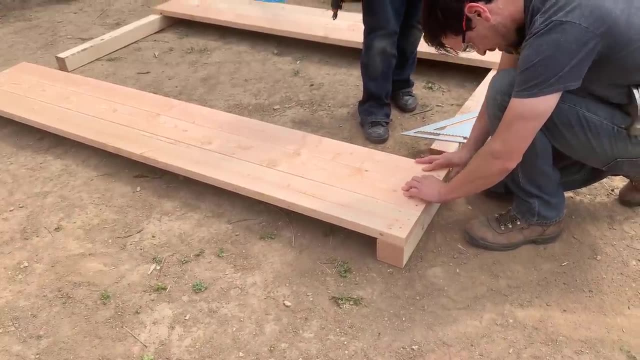 You know that gives us about sixteen and a half inches, because two by six is about five and a half. That seems to be a pretty good height. We're going to fill that with planters mix And then we don't have to bend over too low to get in there to check on the plants and or to weed it. 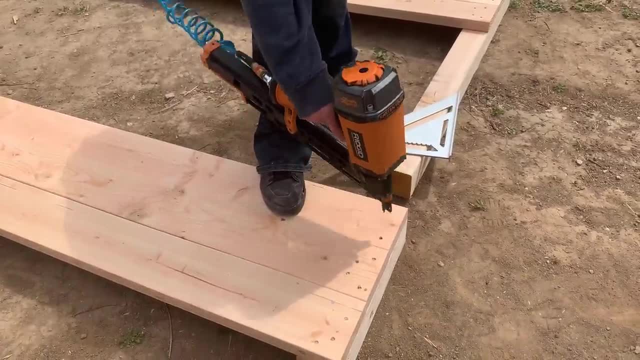 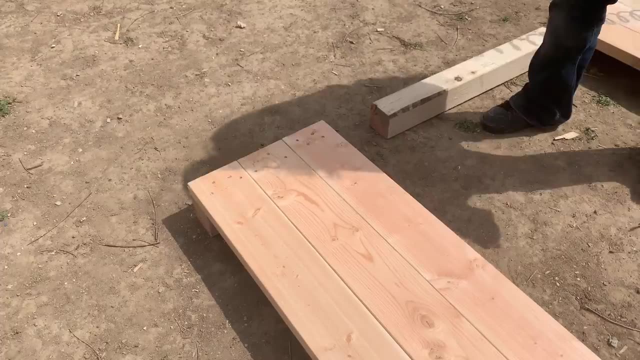 And it's not going to be so tall that we can't reach the vegetables off of the taller plants like the tomato plants and stuff like that. I know there's a few debates out there as to whether or not pressure treated lumber is safe for vegetable gardens. 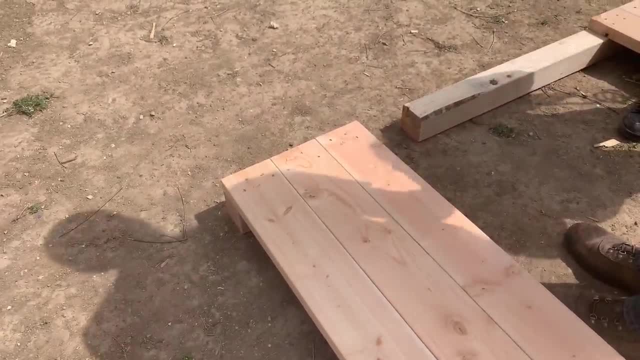 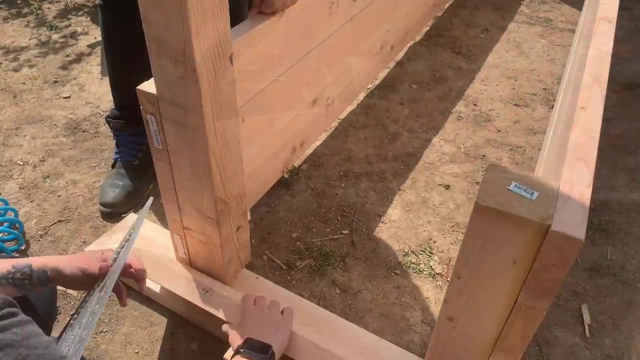 And I'm not really going to get into any of those debates, But I'll tell you that I am a chemist- It's what I did for most of my life- And I'm not at all a chemist And I'm not at all comfortable with putting plants in here that we're going to eat that have been grown in pressure treated lumber. I know for a fact the chemicals from that will leach into the soils. And I know for a fact some of that will be drawn up into the plants. Exactly as to how much, I don't know, But I'm not going to have that. 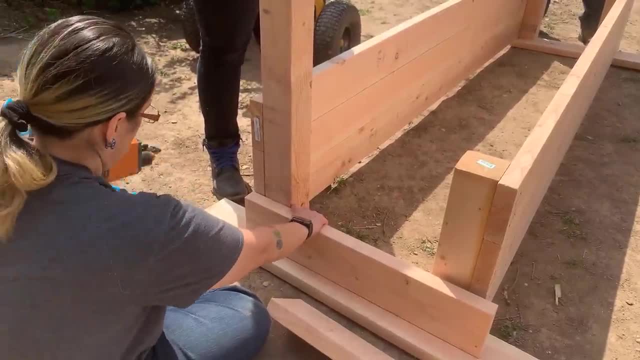 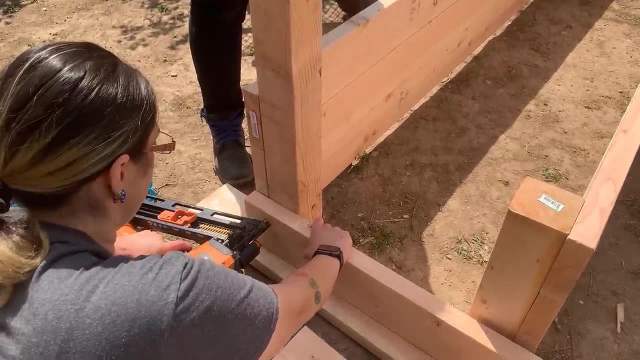 I would rather use plain wood, whether it be something like this Douglas fir or southern yellow pine, Or, if I want to spend more money, I would go with cedar Or something, or redwood, A wood that has a higher tannic acid that's not necessarily going to rot or decay. 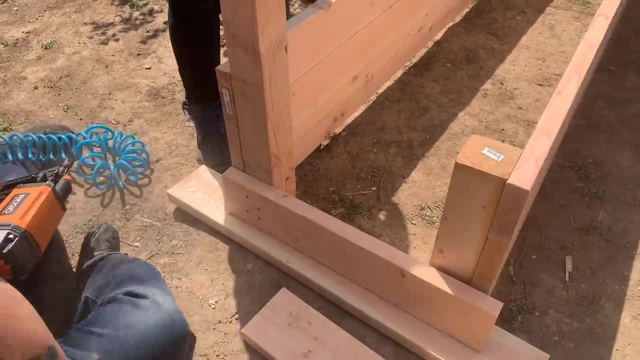 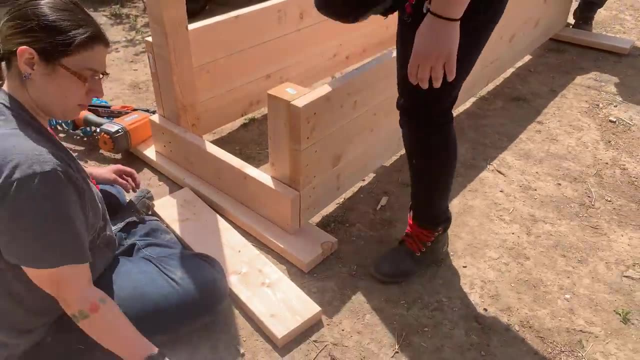 But I would never use a pressure treated lumber for anything that I build Here. Maya is nailing the ends onto the two sides, the two long walls of one of the planter boxes. You can see that one of the long walls has got tall 4x4s. 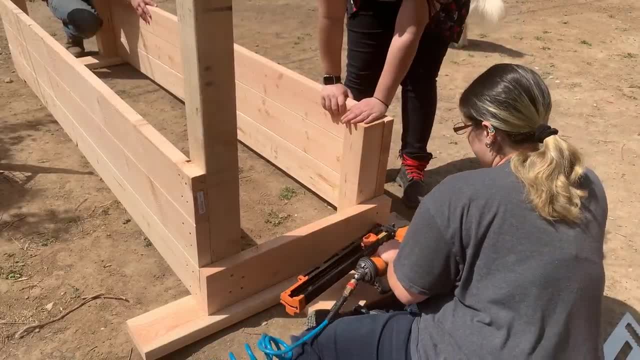 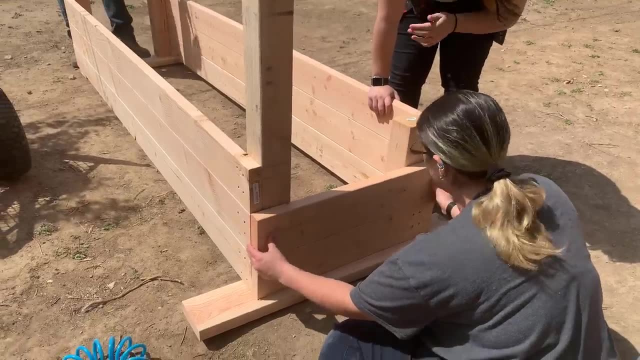 That's where the fence is going to be on that section And the inside of course has short ones And it's going to be the same thing. So a little 2x6 laid horizontally there at the bottom to get a nice flat surface. 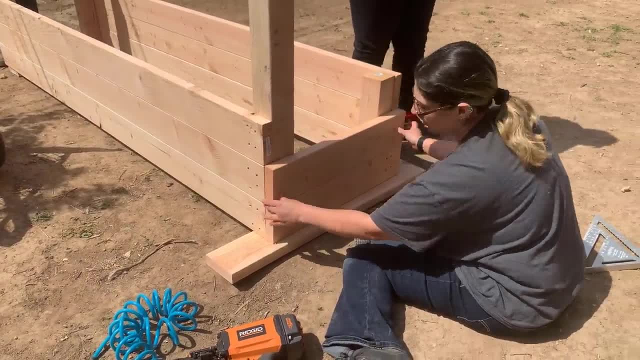 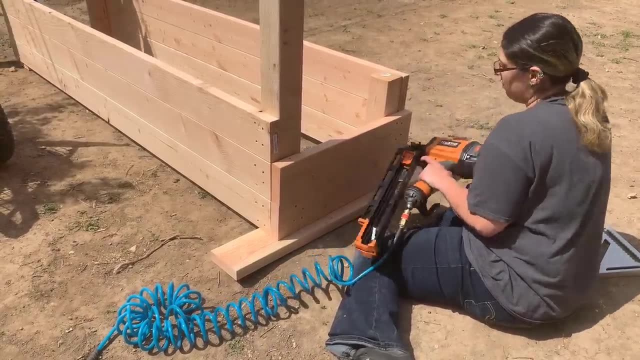 So that we can make sure that the two sides are perfectly flat on there, And that just keeps the box build relatively square, Since the ground, of course, is a little bit uneven. The other cool thing about this project is it can really be done with a very minimal amount of tools. 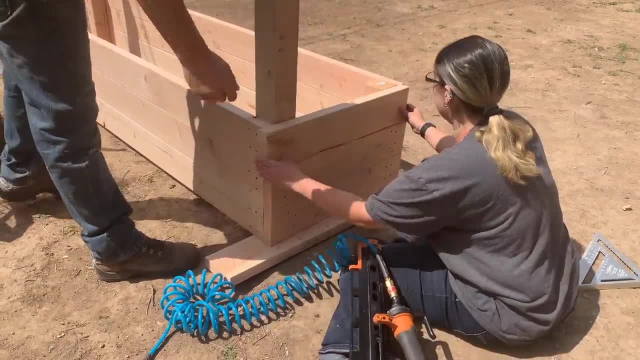 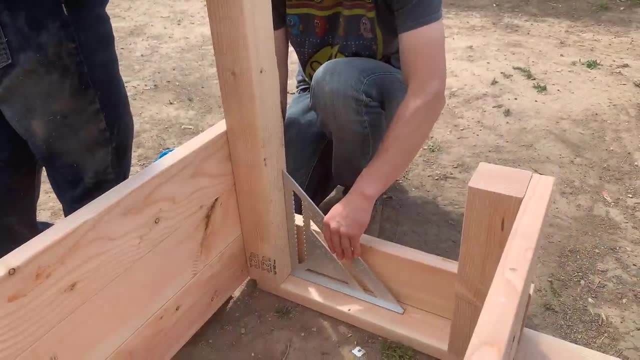 You certainly don't have to have a nail gun. You could drive screws in here, Or you could simply hand drive nails. That would work just as easily, And that plus a circuit breaker, A circular saw And a square- Something like this rafter square. 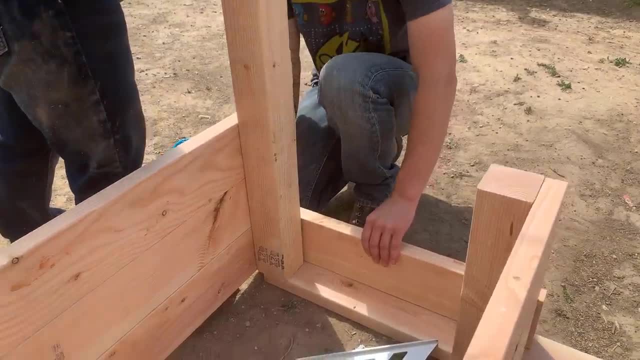 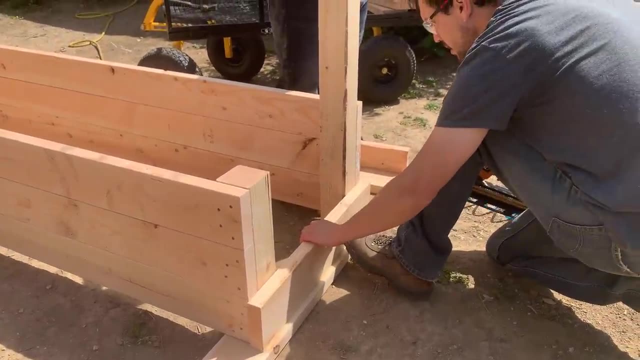 Is really about all you need Here. you can see they're doing the other side And you can see that 2x4 laid flat on the bottom, Or 2x6, sorry- Laid flat on the bottom to give us a nice flat surface. 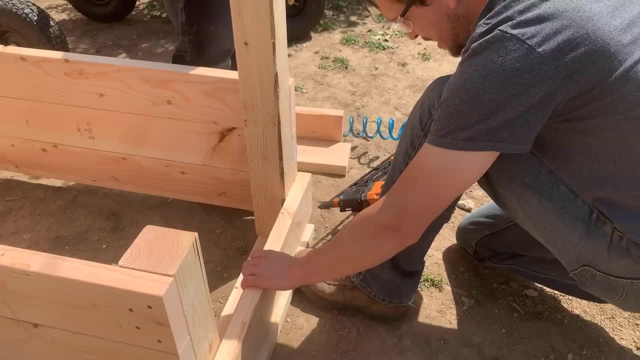 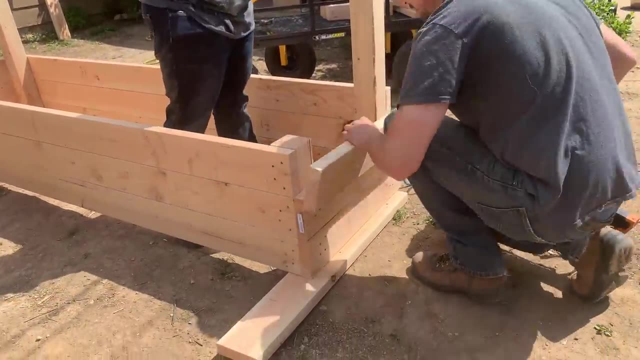 To start our first vertical 2x6 there, And we'll do the same sequence here. We're just going to build up three 2x6s on this side as well, And that's really all it takes to complete one of these boxes. 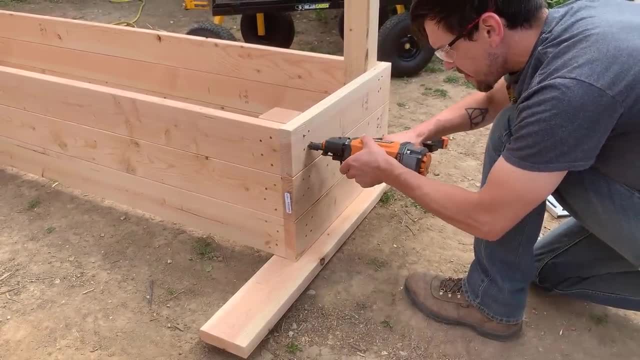 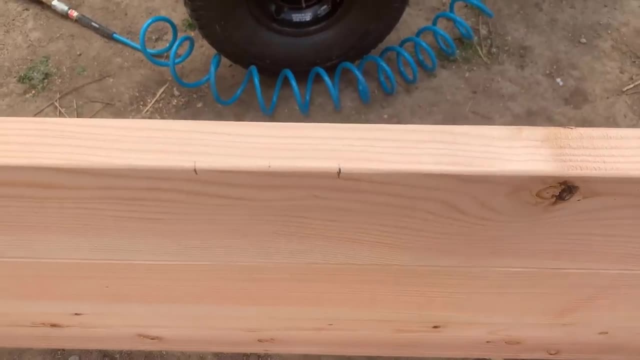 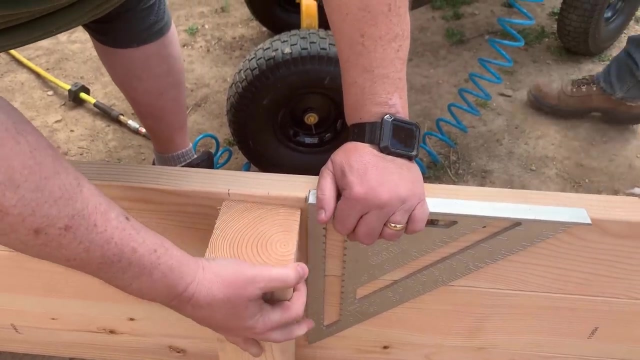 We did do one additional step here. I've located the center of the box, I've kind of marked out a spot to put a 2x4 on And I'm going to Or a 4x4- in this case A 2x4- or a 4x4.. 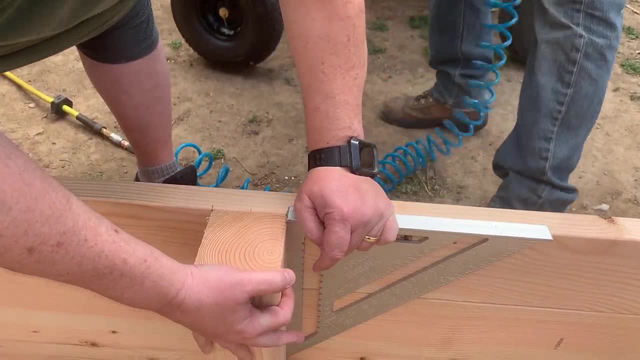 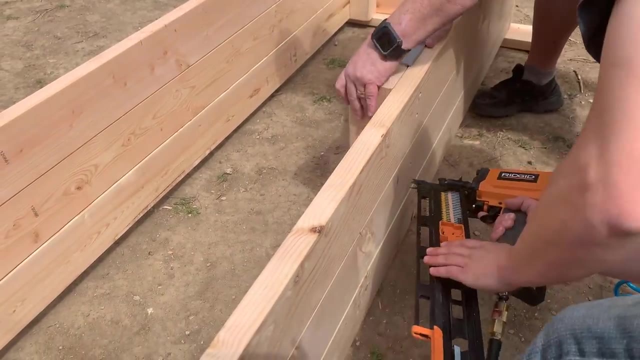 Either one would work. I just used some scrap lumber in here. We're going to affix this to the sides, One on either side- And then we'll put a board between them In order to proceed, In order to prevent these walls from pushing apart. 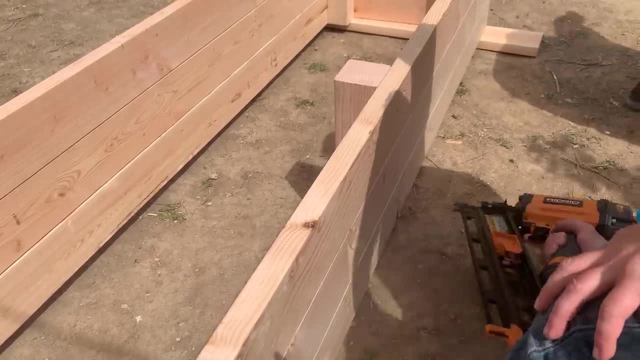 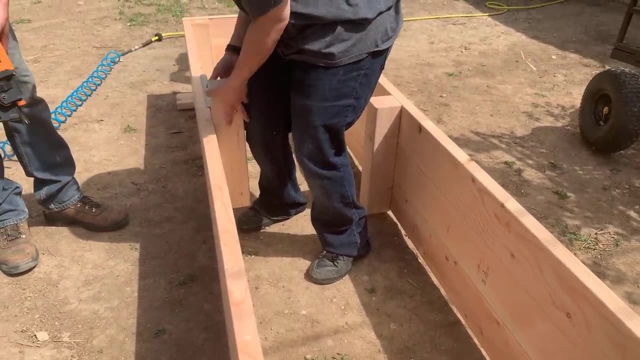 Over time. I think that these walls would probably stretch a little bit Or be pushed out a little bit Once it's filled with dirt And the pressure gradually builds up. I don't think it would happen for a couple of years, But we're going to put this in here so that this lasts a little bit longer anyway. 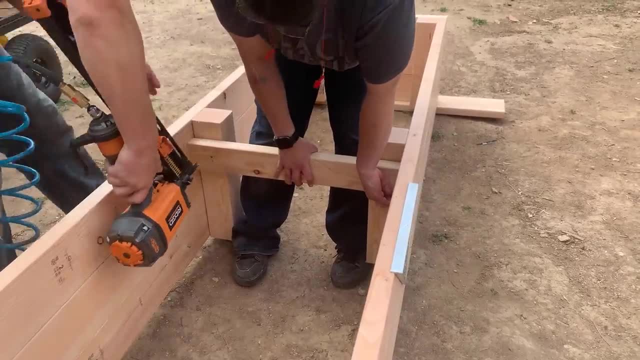 And you can see the 2x4 there that we're putting across And that's just going to kind of help hold this box together in the long run And it really doesn't take up that much space on the inside of the box. 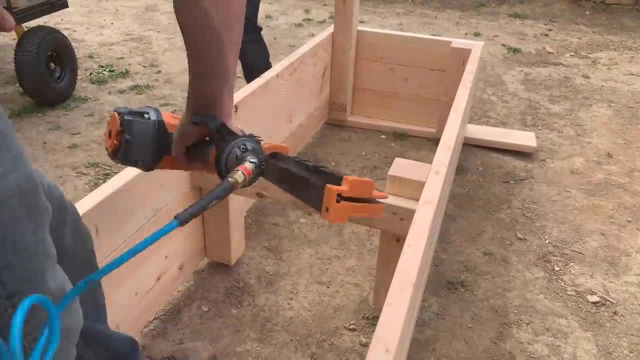 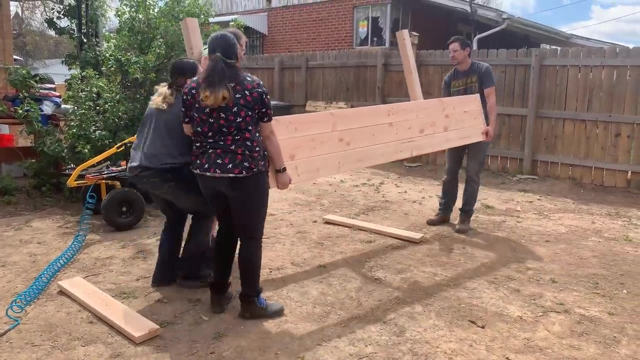 So it's not really going to take away from your planting area too much. We're still going to just fill the whole box with planters mix anyway, And once that box is done, We're going to just carry it in place. It might have been smarter to build it in place. 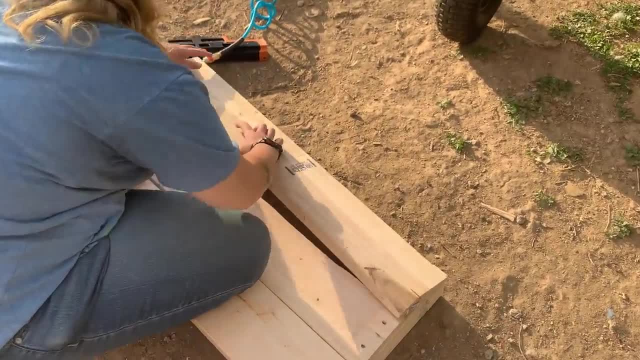 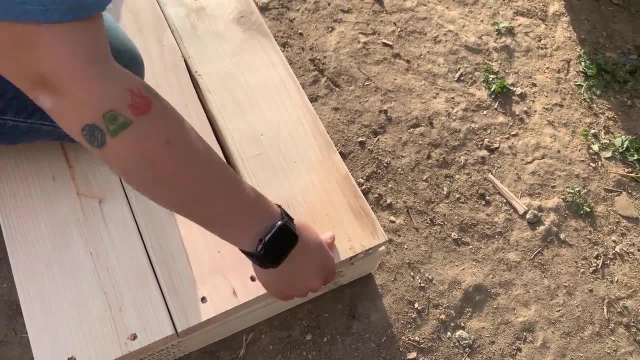 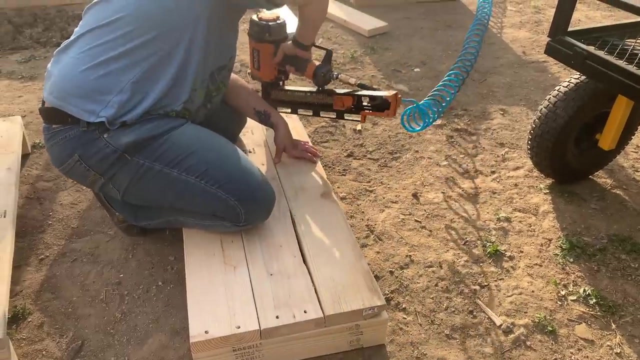 But you know, we didn't really think that far ahead, of course. And here Maya is building the shorter wall sections Which are going to go between the main planter boxes To kind of fill out the overall shape. And before I forget, I wanted to take a moment to ask if you enjoy our channel. 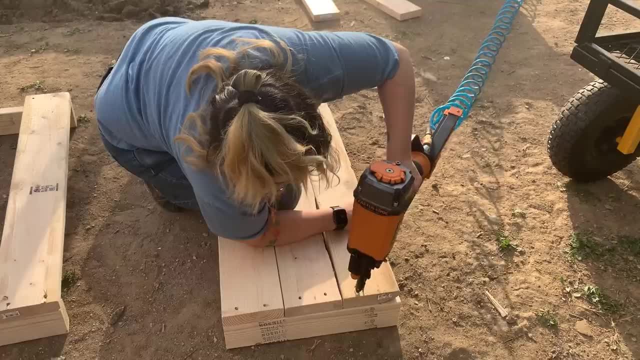 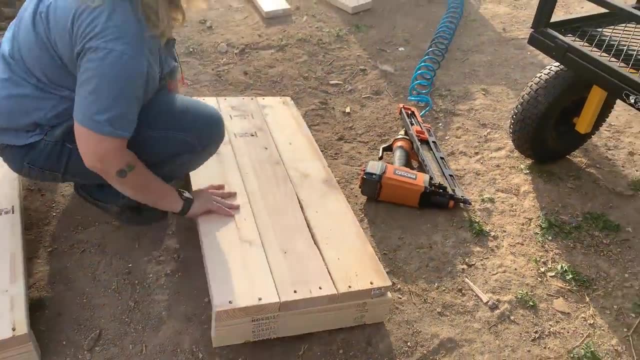 And the videos that we put out. If you would just take a moment to click that subscribe button down below. It's how we grow and we really appreciate the support. You can see where they're going to go here. She's going to put them between 2 planter boxes. 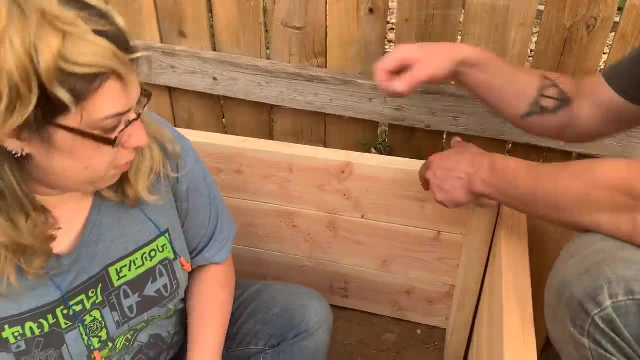 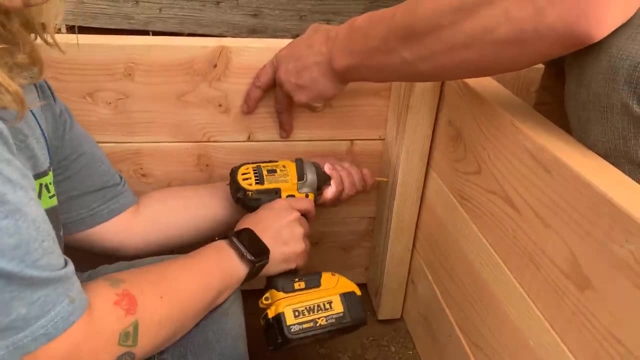 Which are oriented over against the back fence And it's going to fill in the area. We're going to put one right there And one about 2 feet forward of that point And kind of create a line And create another little planter zone in between. 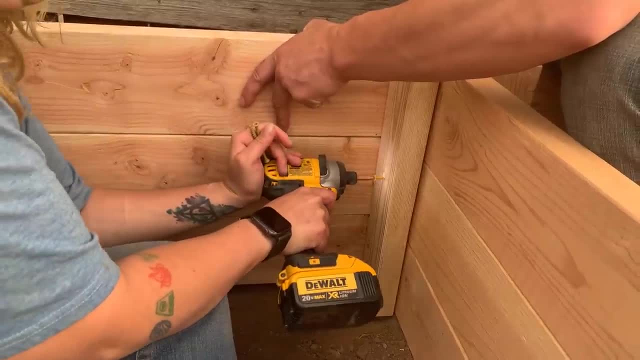 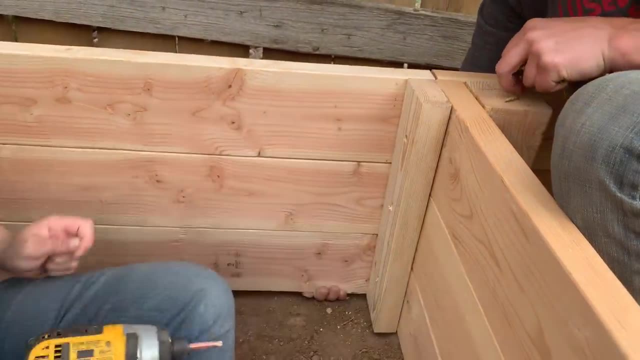 And you'll kind of get a feel for it When it all comes together And you see how it all looks. And this part she's going to screw together Because in the future we may decide to relocate this planter box To another location. 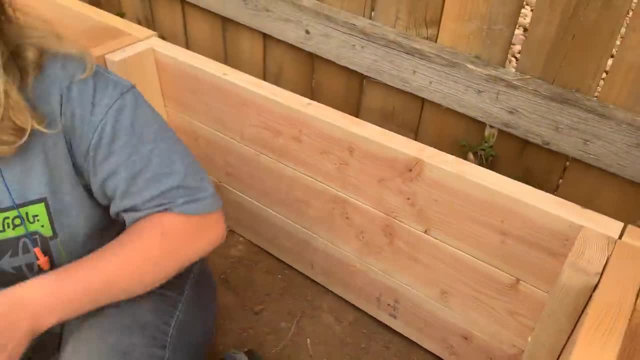 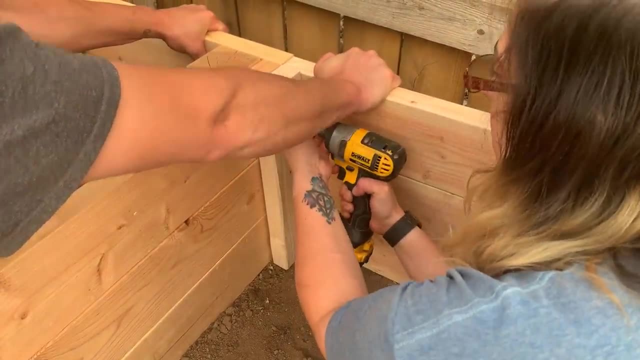 The raised bed garden itself, I suppose I should say To another location, And it would just be easy if we could pull these individual walls out And then move the planter boxes themselves separately. After we installed our shed last fall, Our whole backyard. 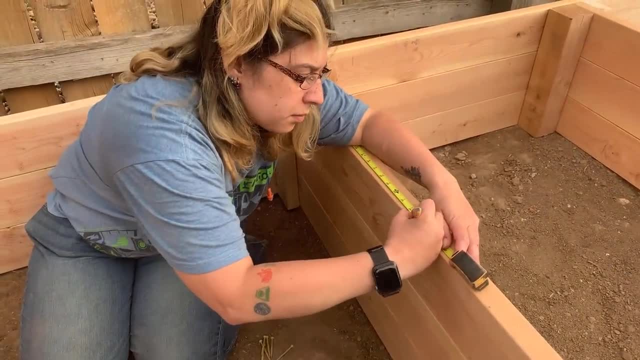 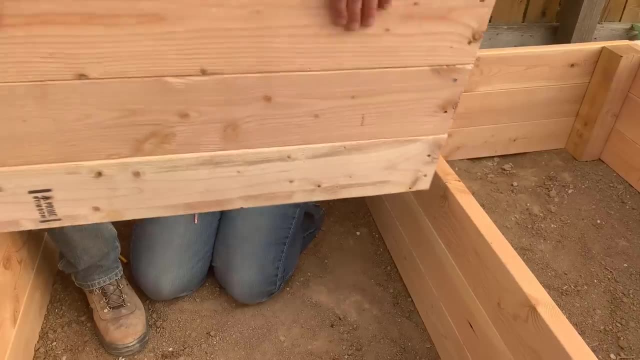 Has been kind of in a state of disarray, And we cut out a lot of the rest of the sod. We're planning on doing a complete re-landscaping of the back, And so that's why the possibility exists That we may move this raised bed garden. 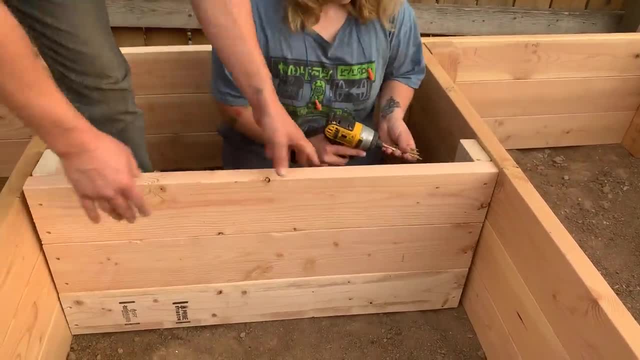 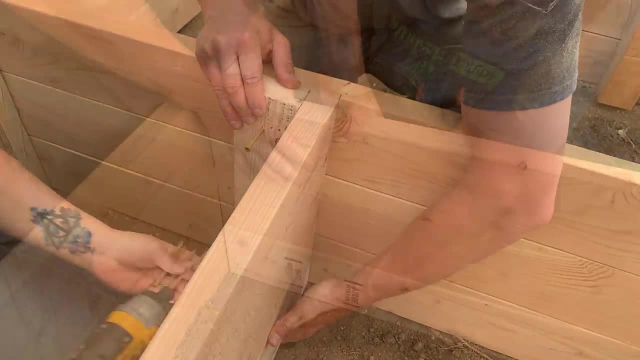 I think it's going to probably be here, But in the event that it's not, It'll be easy to disassemble and take the boxes elsewhere. And you can see this is the second wall, That's a little bit in front of that first wall. 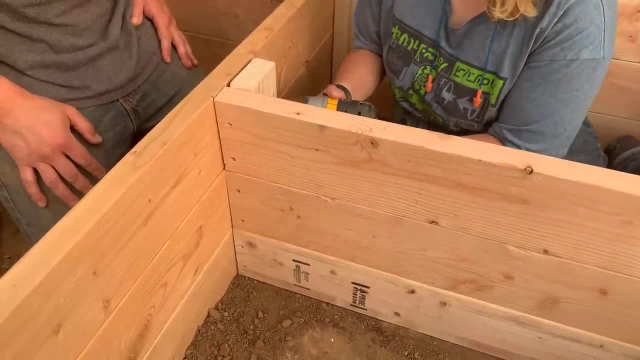 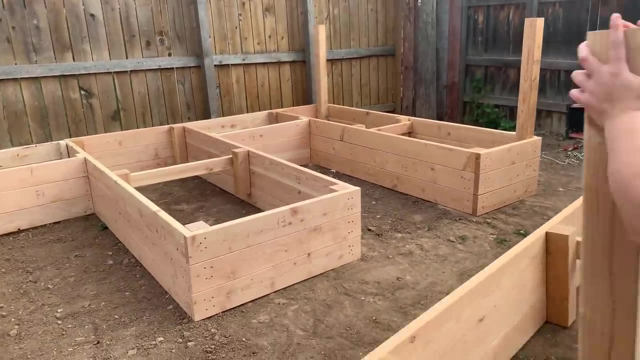 That's going in here And that's going to be a portion of the raised bed garden as well. Hopefully here you can get a little bit of a sense of how that's going. You can see the little short walls in the back That are kind of attaching those three main planter boxes together. 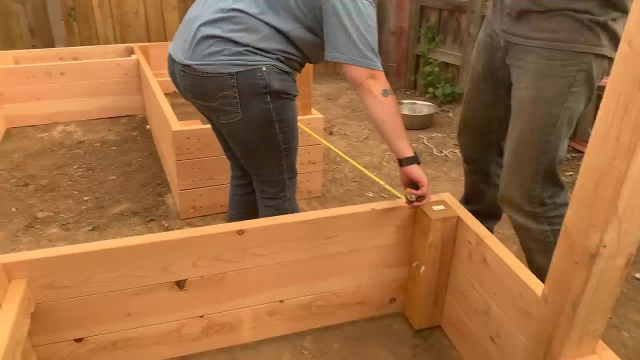 And then we've got a front planter box That we're turning at an angle 90 degrees to the back one. We're going to put a little short wall in there too, And all those intermediate spaces in between Are going to be walking areas. 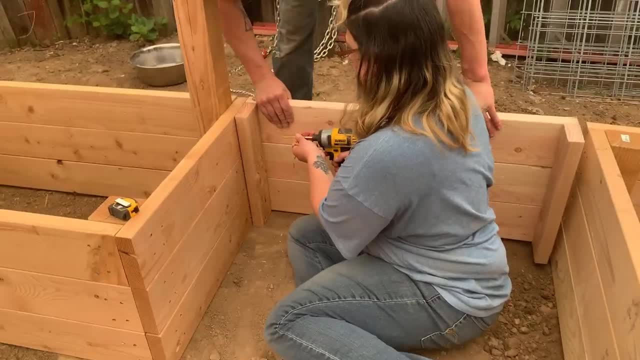 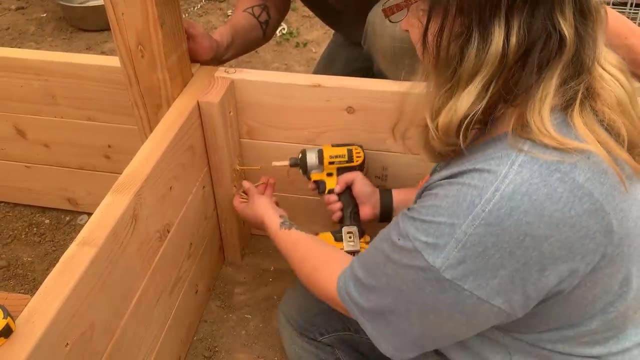 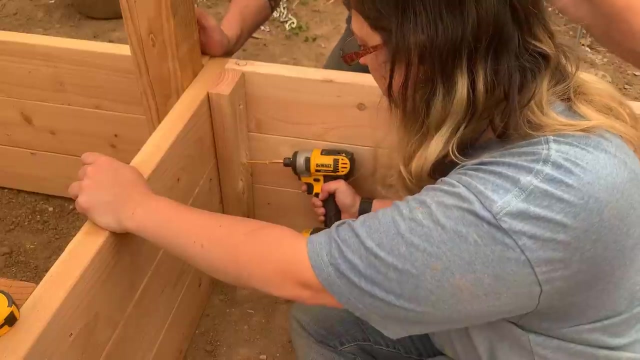 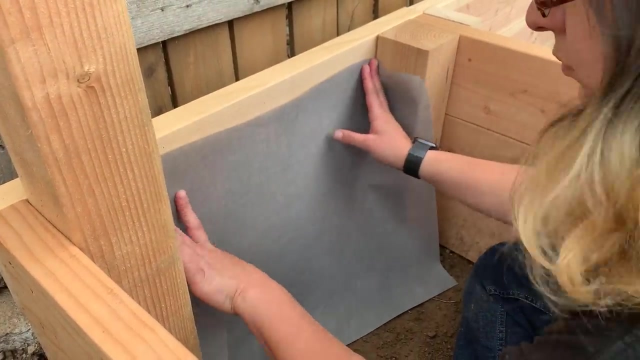 So we can walk in between each of these separate sections And easily access the garden area. Once those are all up, We are going to install a landscape fabric, Basically on the inside perimeter of the walls. Well, the reason we're doing this, 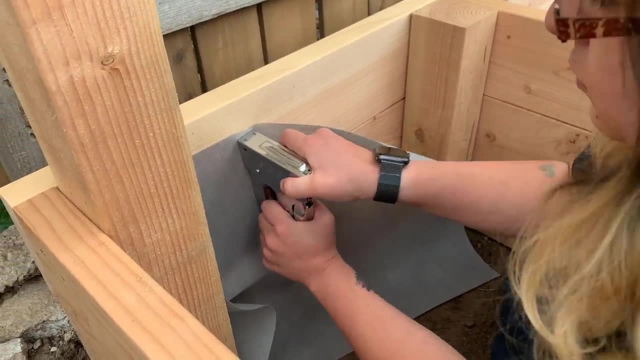 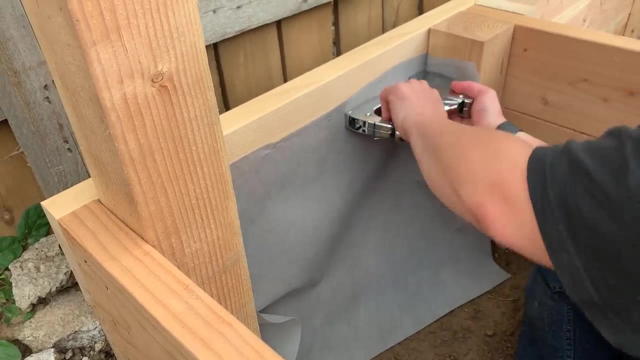 Is not so much to prevent the walls from staying in contact with the dirt, But mostly so that the dirt doesn't pour through the walls. When we water the garden And it turns muddy, Some of that mud might tend to leak through the gaps in the 2x6's. 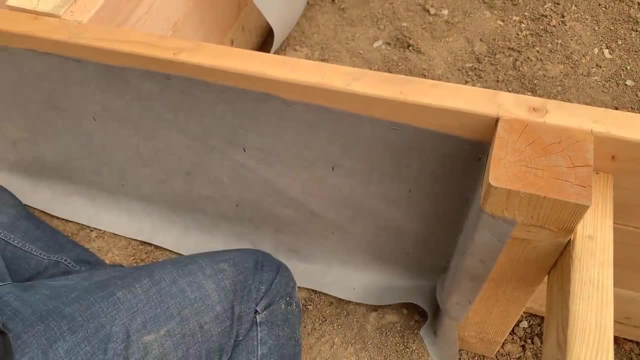 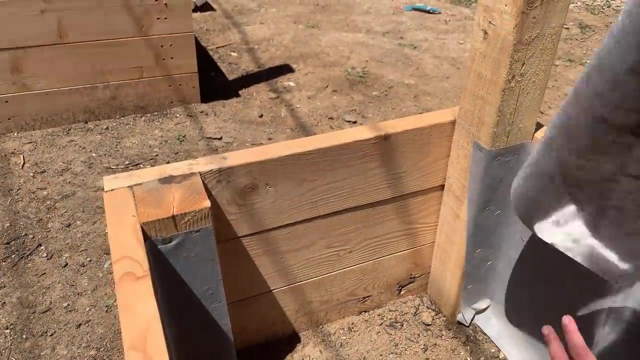 Especially over time when the 2x6's shrink a little bit And then the outer portion of the walls would look pretty ugly, Especially if we have a nicely landscaped yard. And this is just going to prevent that from happening. We won't put any landscape fabric down in the bottom. Because in the event that we have any plants that have very deep roots, We still want to have soil down there For the roots to go ahead and access that area as well. It does have the added benefit That it will probably slow down. 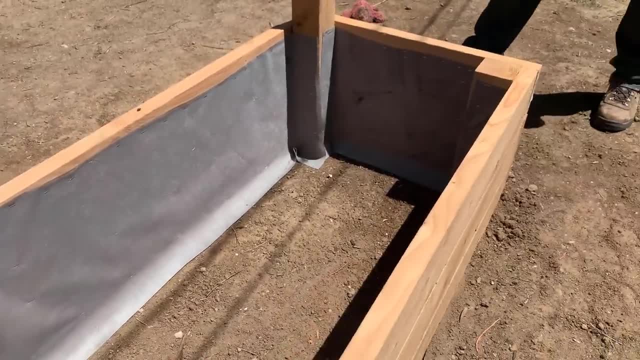 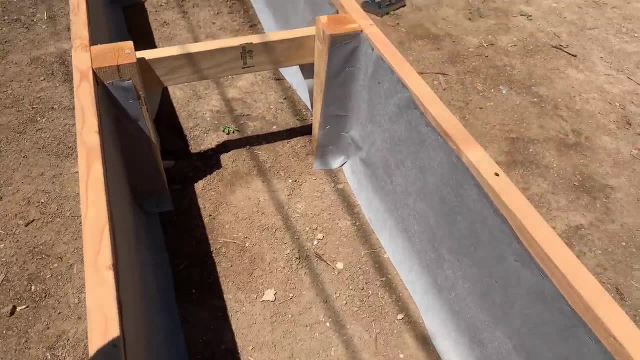 Some of the rotting of these 2x6's. But here again the main purpose Is just simply so we don't have dirt or mud Escaping through the joints Or the gaps between the boards Once those were all up. 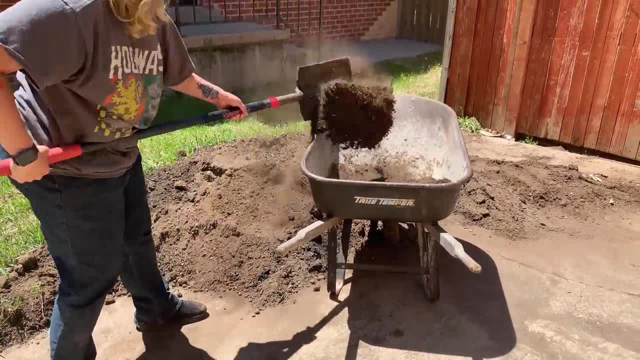 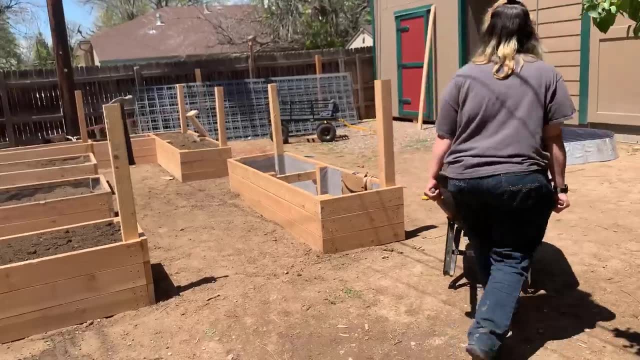 We ordered a few yards of planters mix, Which is a combination of topsoil, peat and manure, From a local garden center And they delivered that for us And we're going to go ahead and fill the boxes. You can see right there at the front. 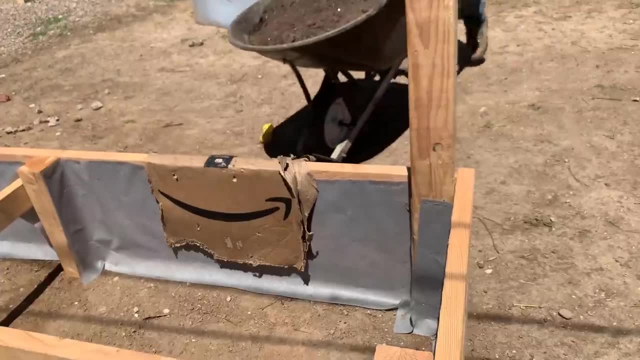 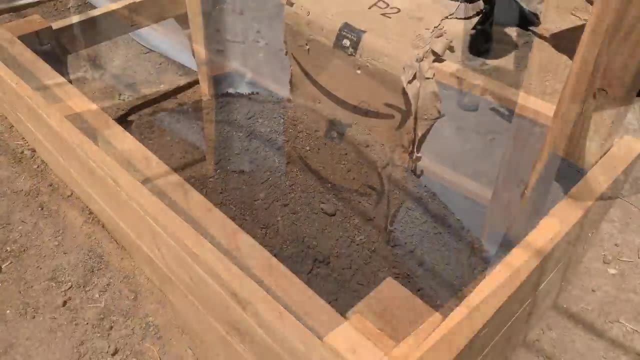 We have a short section Where we don't have the wall in place, So that we can get the planter back there a little bit quicker. We'll put that in right. at the end They put a little bit of cardboard over the top. 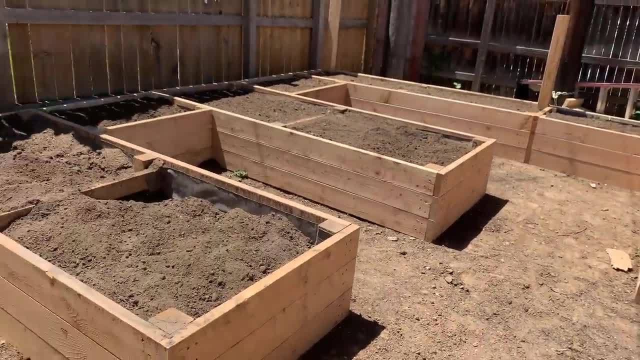 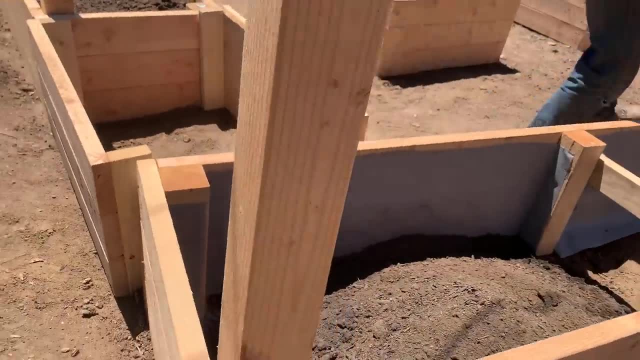 So as not to chunk up the edge of the wood there. But this is what it all looks like. So you can see our walkways are clearly defined, Alright, and we're going to fill up this last area Here now. finally, That most of the planters have been filled with dirt. 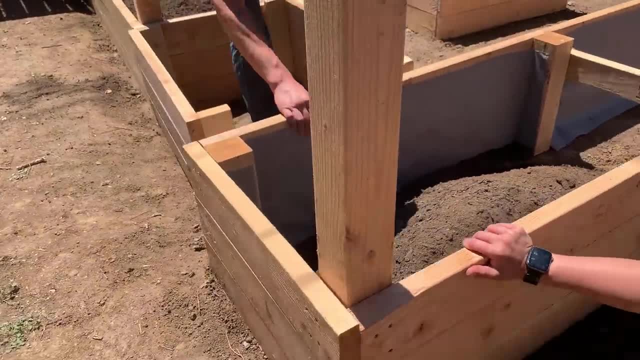 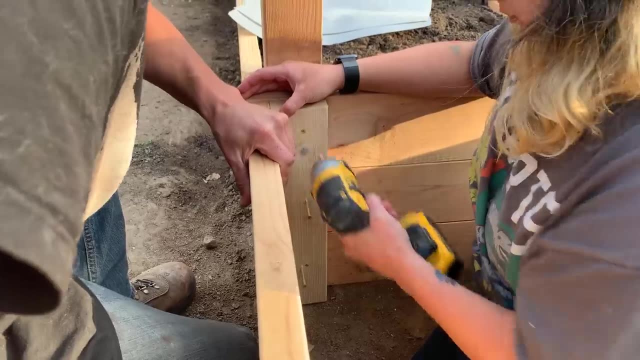 Of course, this might have been smarter Before we put a little bit of dirt in here, But I think we thought it was a little closer Than it really was, And these are just going to be the last two walls That go into place. 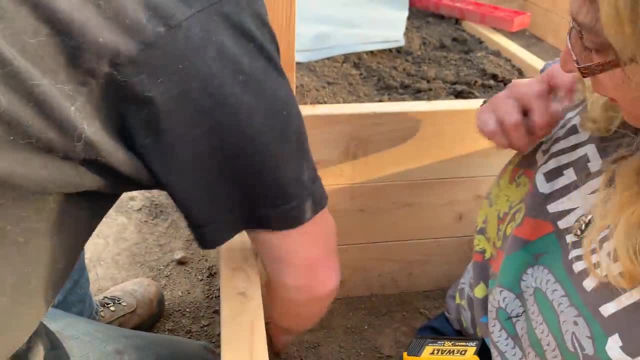 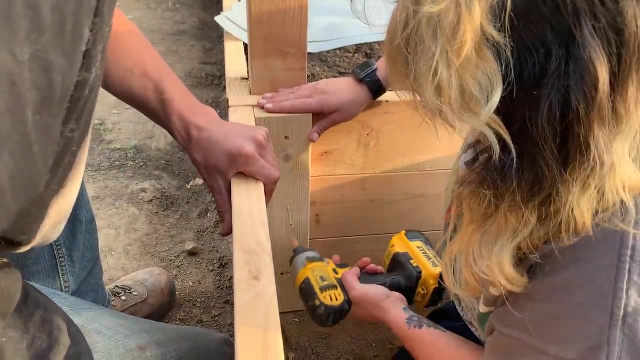 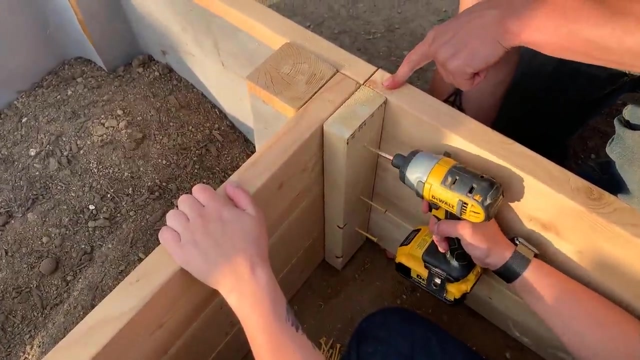 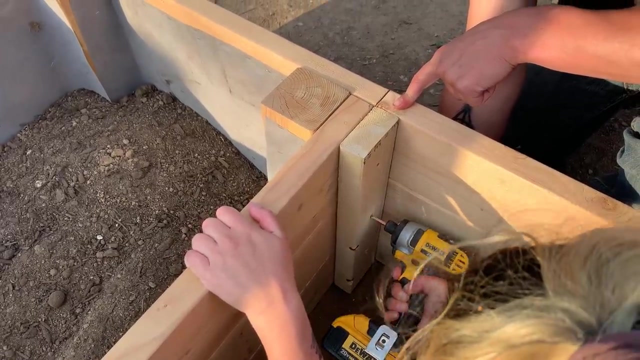 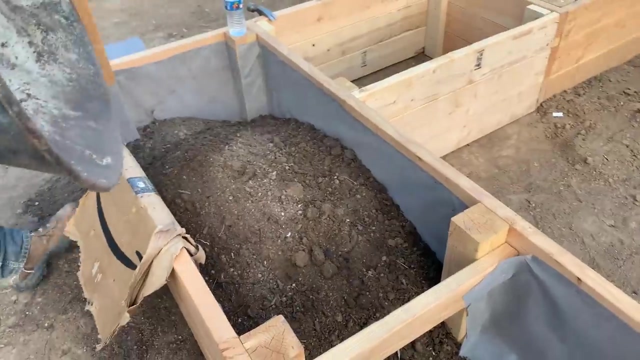 And that will finish off the entire planter structure. This will also help complete the border Around the entire exterior To allow us to get a fence On the perimeter easier as well. Okay, so once these get filled with planters mix, There is one more thing we are going to do. 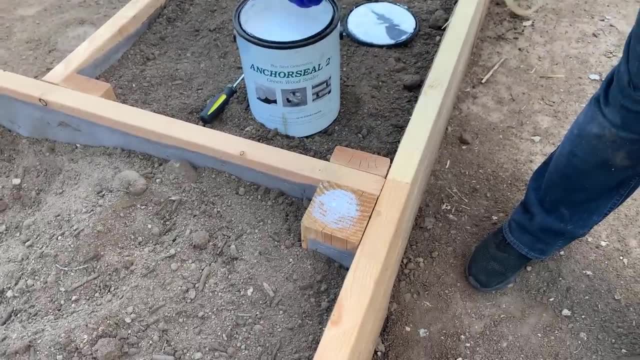 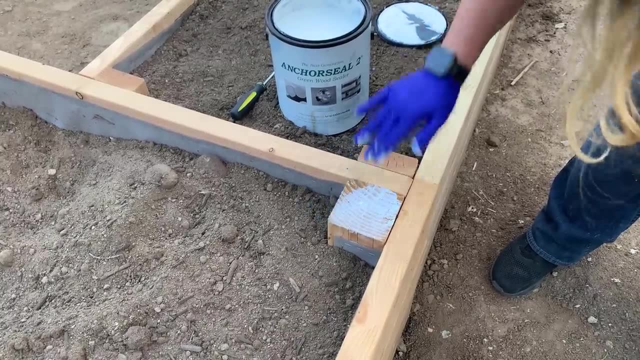 To try to protect these just a little bit. Just on the end grain of the tops Of the 4x4s and 2x4 posts I'm going to put anchor seal. You could also put latex paint, Something like that, on there. 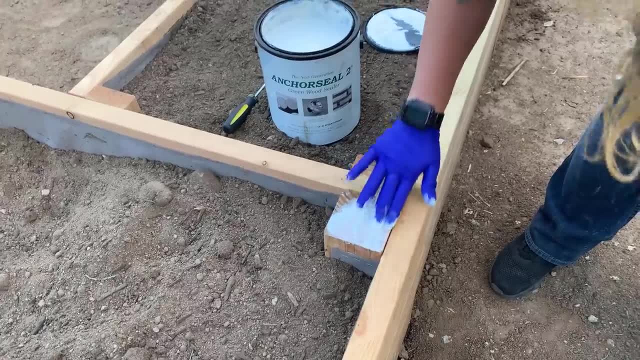 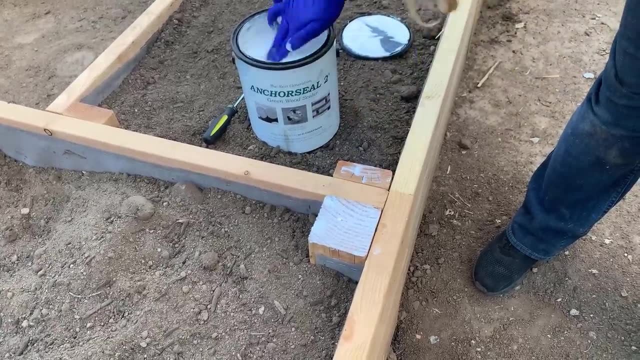 What that's going to do Is it's going to stop the draining water From just soaking down in there And disintegrating this really quickly. It's going to. If we don't do this, It's going to splinter and chunk up pretty fast. 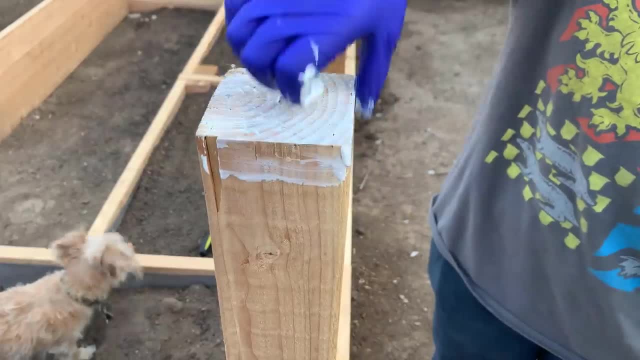 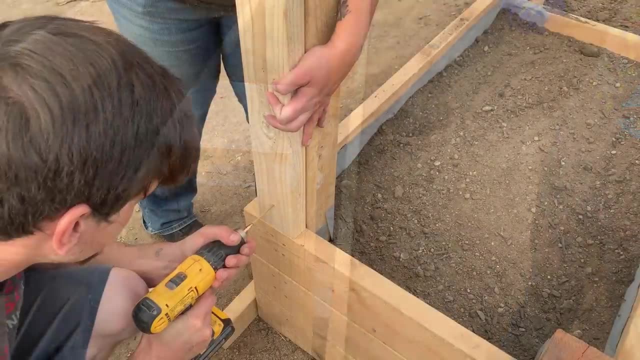 Probably within just a few weeks or a few months, Which might affect the integrity of it. It might not, I'm not really sure, But I know by doing this It's going to allow the posts to have a considerably longer life span. 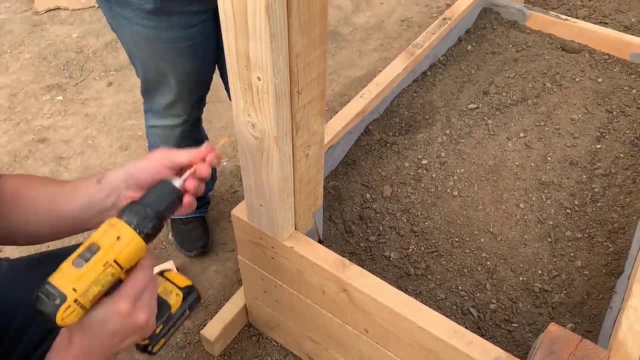 And they'll end up lasting just as long as the rest of the 2x6s. So now, working at the entrance to the planter garden, At the area where the gate is going to go, We're going to put some 2x4s. 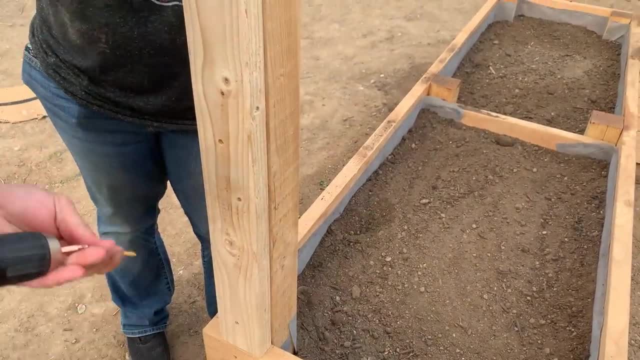 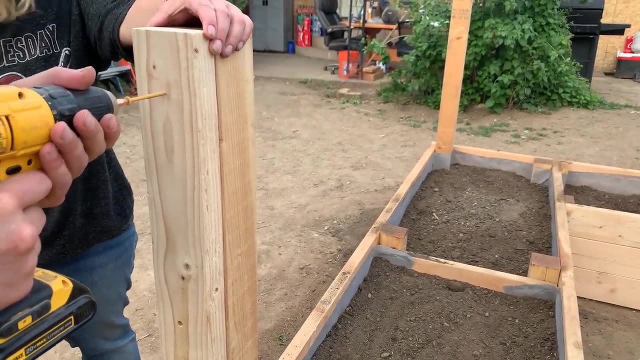 And some 2x6s To flush out this, The post. to get it out to be flush With the 2x6 wall. It's going to allow us a place to attach the gate And on the side, The inside there. 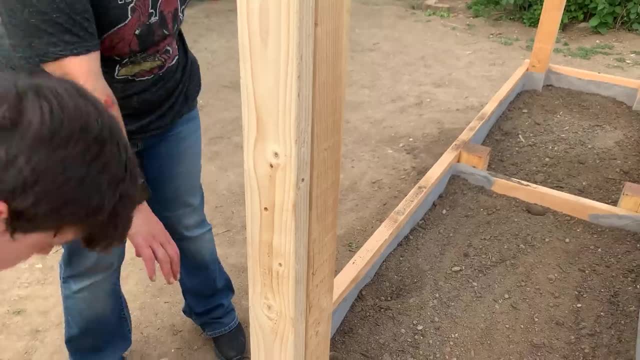 And it's going to allow us a place to attach the fence on the front. So on the inside portion here We're going to do a 2x4. And then we'll just grab a 2x6. When we come around to the front. 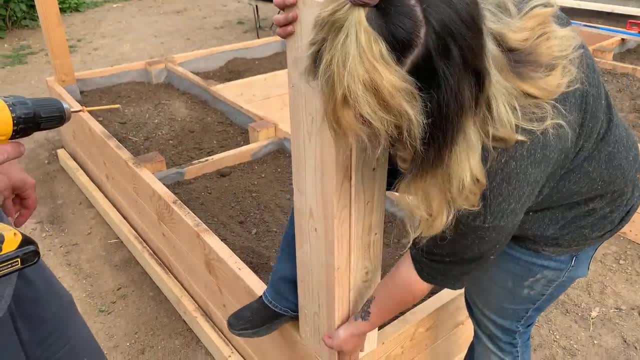 And you can see that's going to look a little bit nicer. It's going to square up that corner a little bit. This is the left side of the entrance, And then, of course, We'll follow up and do the exact same thing. 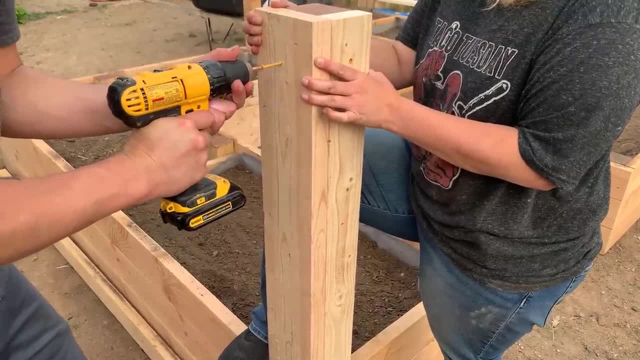 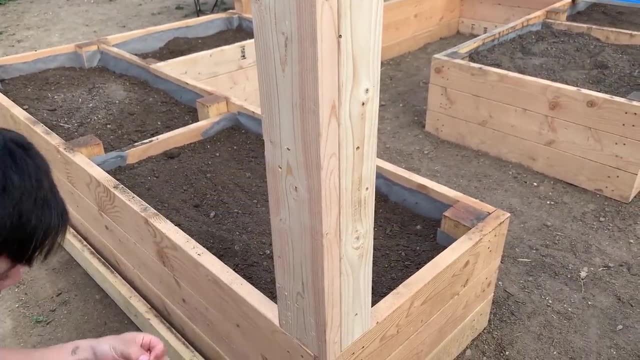 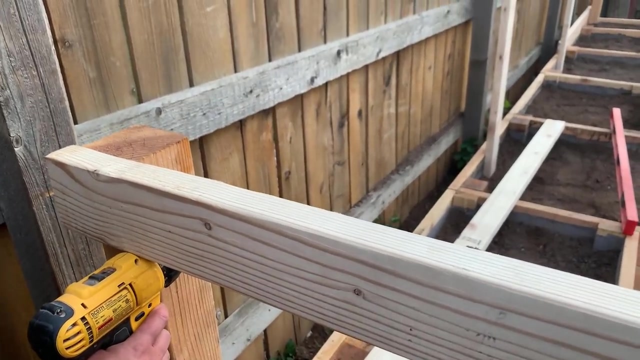 On the right side entrance also. That way there's a location for the gate To attach right in between these two. After that, we're going to jump to the two sides And we're going to just raise a 2x4.. Up to the top. 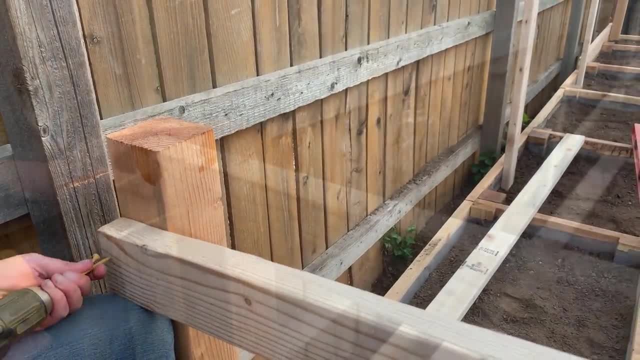 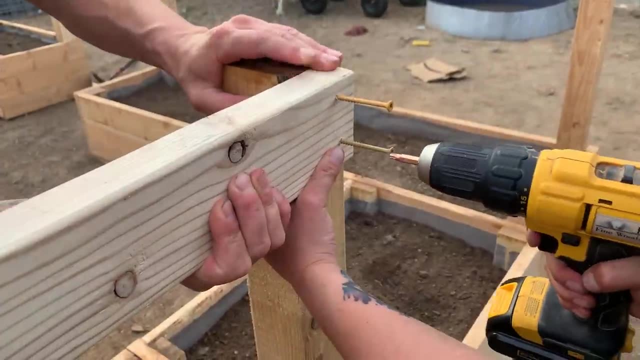 Of that 4x4 post. It'll create kind of a rail That goes across that section, Functioning as a place for us To attach the fence at the top. It's going to end up being flush out, Plumbed to the same distance out. 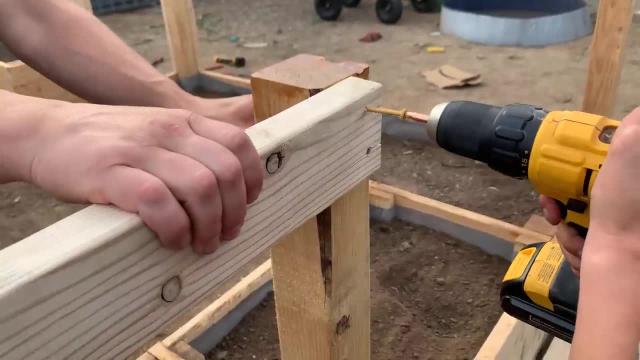 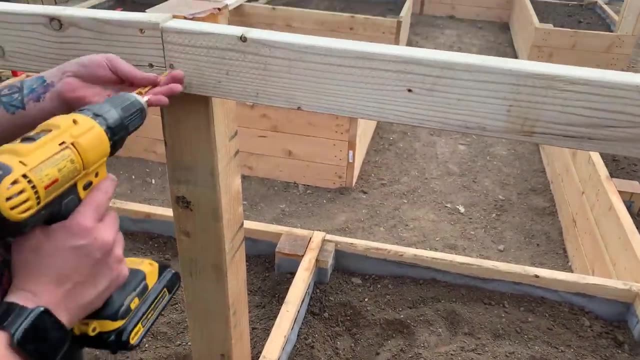 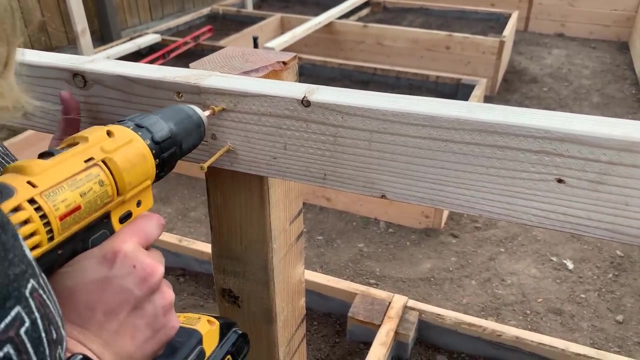 From the post at the bottom, 2x6's are, And we'll split this one right in the middle here So that we can run another short section of 2x4.. On to the end And we've cut this 2x4.. 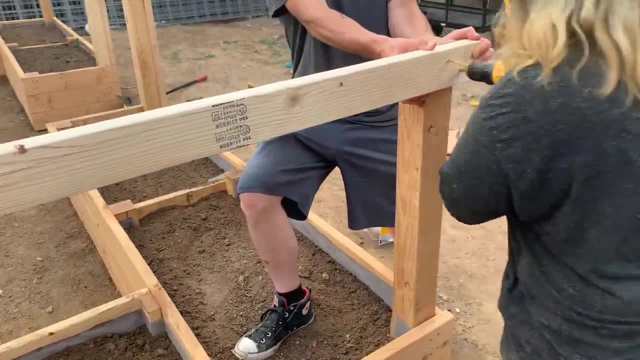 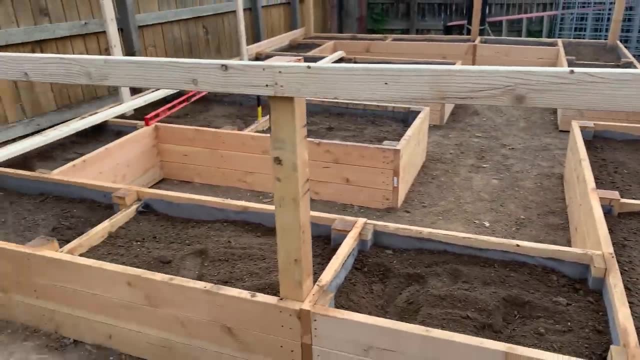 On the right side About an inch and a half long, So it's going to come out flush with the outside Of the 2x4 that goes along the top In the front. That's what the That looks like from the side there. 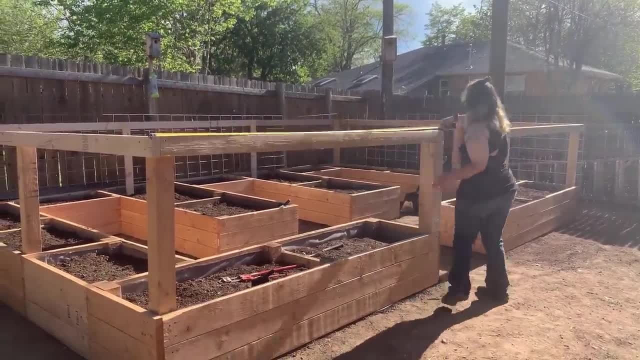 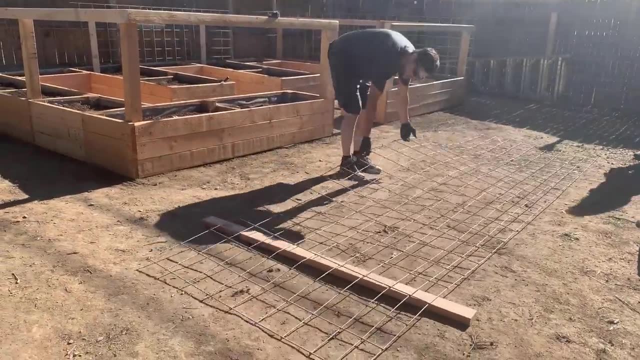 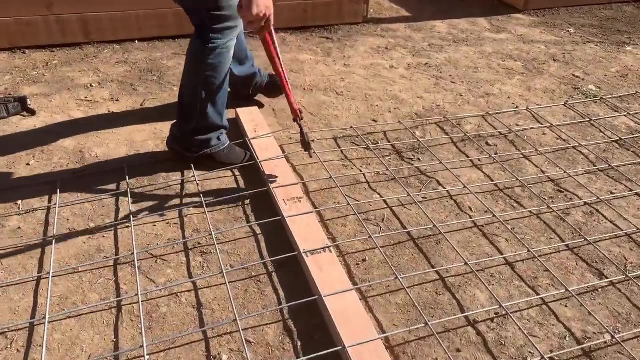 And you can see we've got the ones attached on the front At this point also, And then we're going to Cut our sections of fence next. So this Material is called cattle panel. Now, this Material is very economical And it's very rugged. 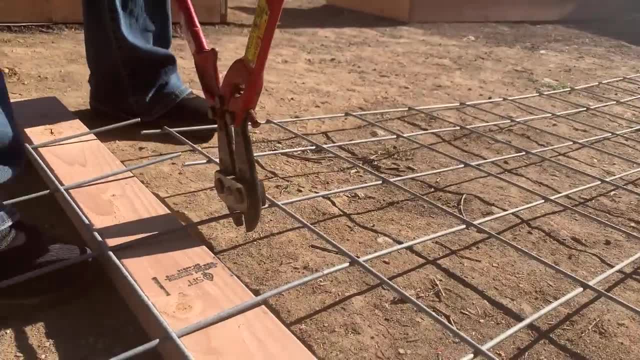 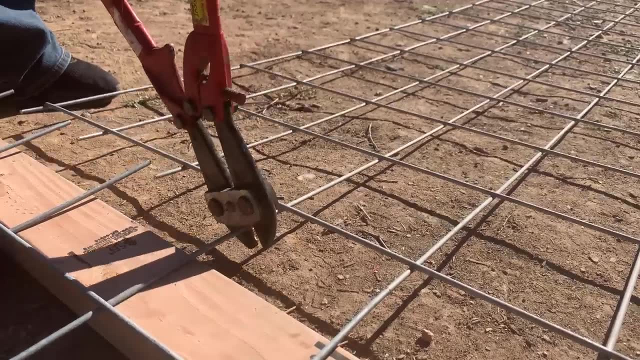 It's a very heavy gauge steel. We got it at a tractor supply store near us- Any place that sells horse feed Or cattle supply Or any tractor supply- And there are also many hardware stores that sell it- And I think we paid around $22.. 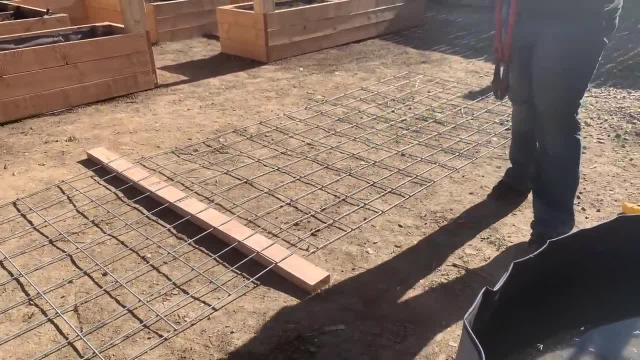 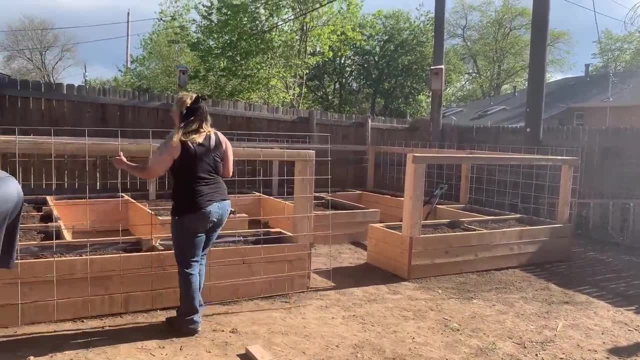 Per sheet for this, And it's actually 16 feet long, So it covers a whole lot of area For not a whole lot of money. I think 4 or 5 sheets or something Covered the whole perimeter of this, So it wasn't really too bad. 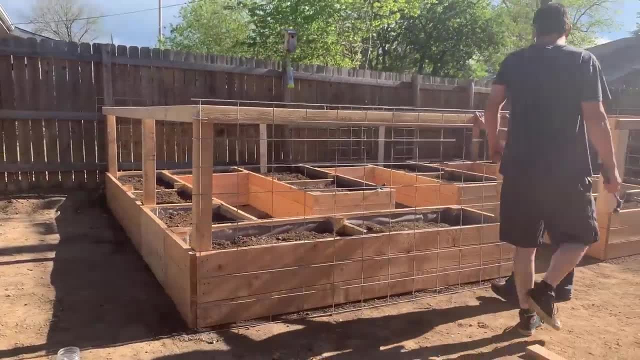 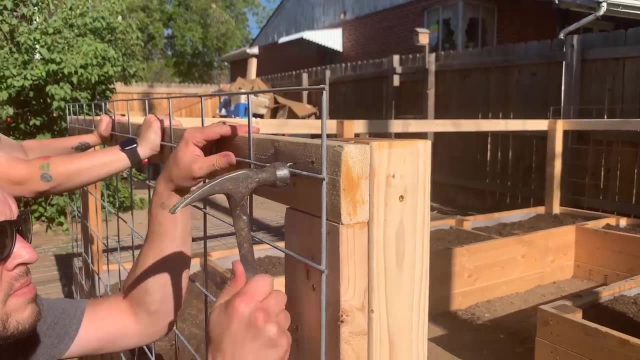 And it will positively keep the dogs out, And I think it's 50 inches wide, So about 4 foot 2 inches wide. Now, a U shaped nail would have been better here, But I didn't have any. We couldn't find any. 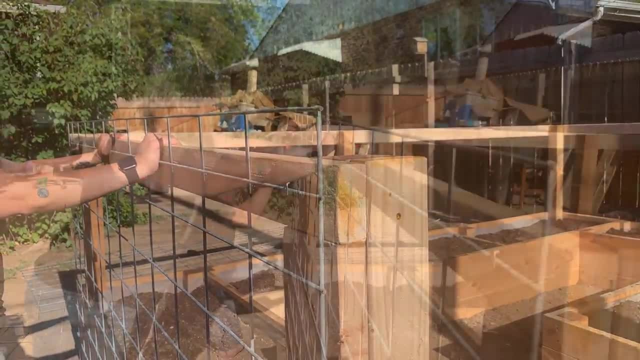 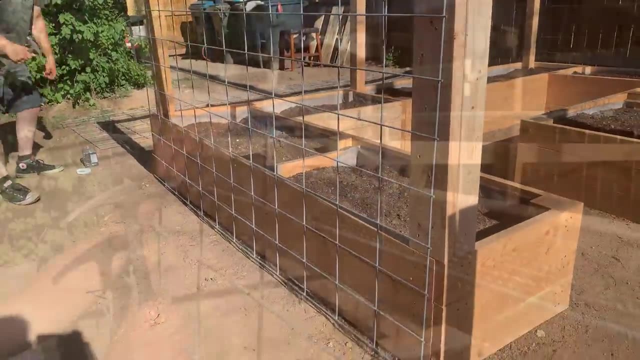 In fact, our local store was out, And so we just put a little square nail, A U shaped nail, Kind of one that holds electrical Romex wire down, And we'll replace those later When we get some U shaped ones in stock. 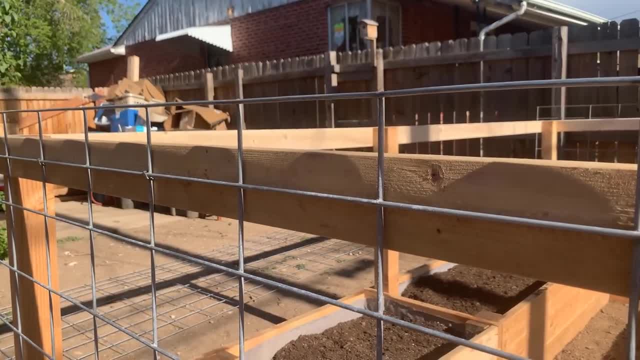 We're going to have to figure out how to do that. We're going to have to figure out how to do that. We're going to have to figure out how to do that. When we were finished with these, We added a few zip ties to the corner. 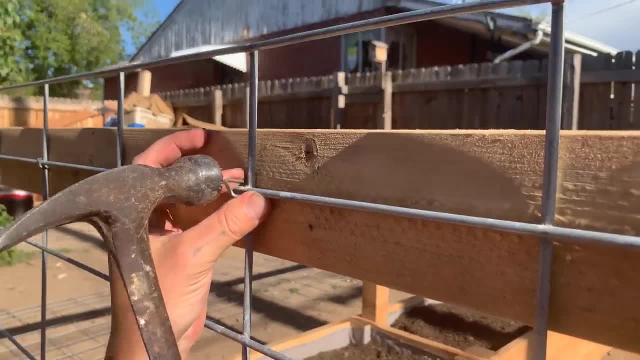 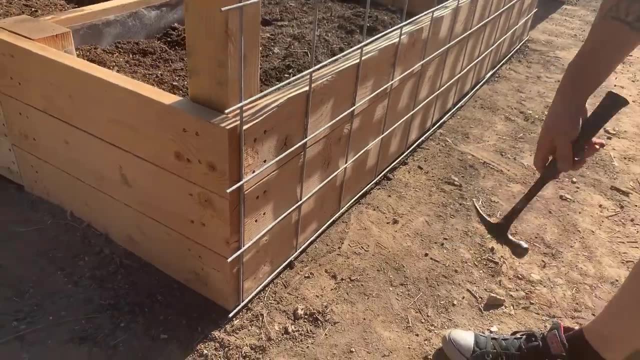 But all in all, we put these about every other joint And they actually ended up holding it really strong. We couldn't pull it out, No matter how hard we yanked on it. So we do plan on replacing them, But I think if you wanted to go with something like this, 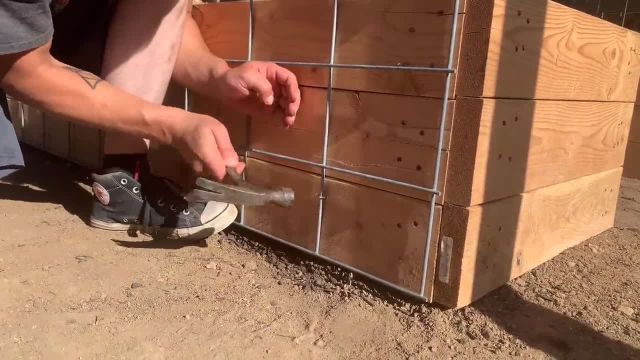 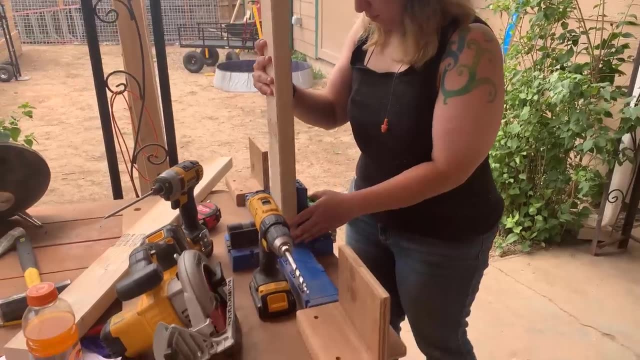 You could. If you couldn't find the U shaped ones, They actually ended up being pretty strong. Next, it was time to build the gate. It's just a really simple gate. It's all made of 2x4's, Just a square frame. 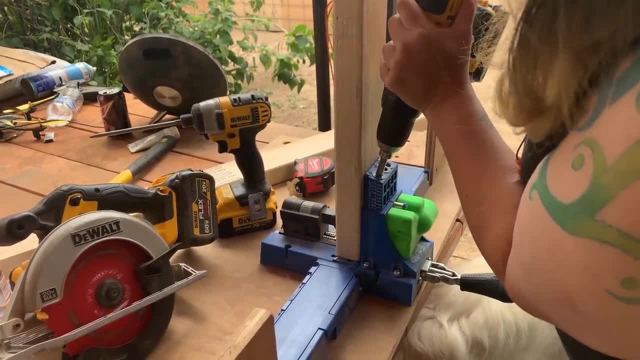 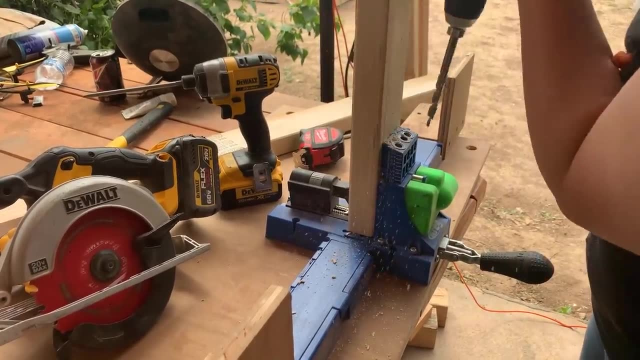 And then an X shape in the middle. We thought the best way to attach it Would be some pocket screws And you can get the exterior rated screws. They're the blue screws. For pocket screws We use a Kreg pocket jig. 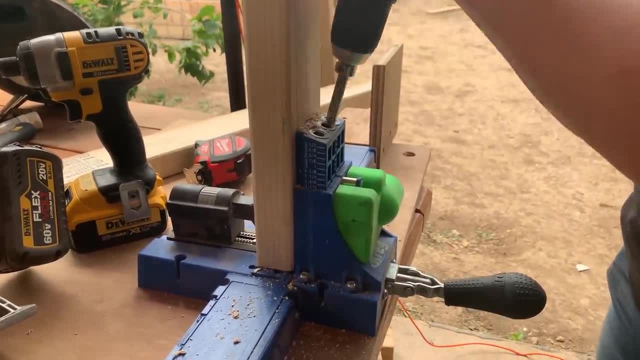 You know. if you're interested in any of the tools That we've used in this video build, I do have a link to all of those in the description down below. You can go down there and check it out. These are actually really strong. 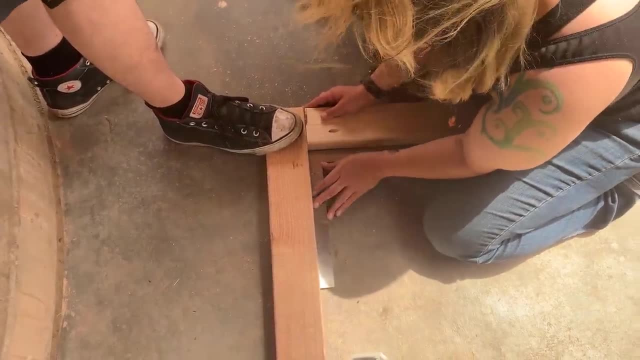 I've got a video on how strong they are in fact. But we're going to put the perimeter of this thing together with pocket screws And then we're going to put the wire On the front of it, And that actually made for a really rigid gate. 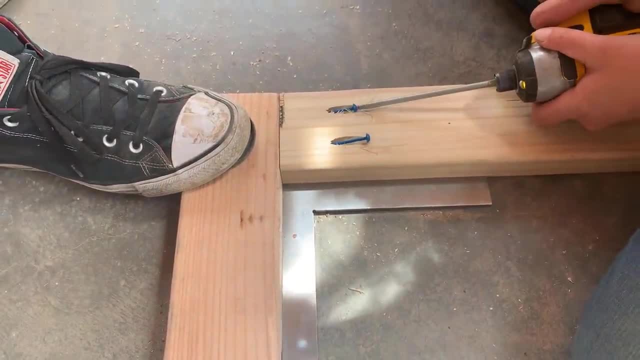 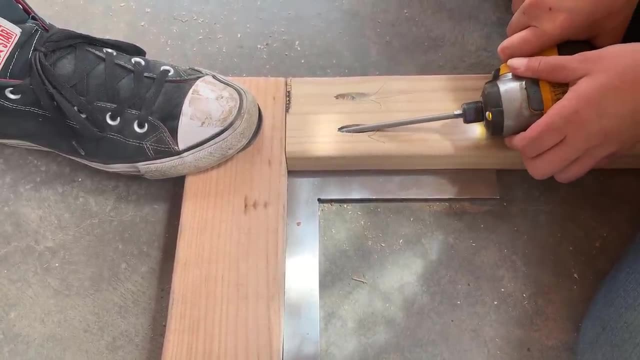 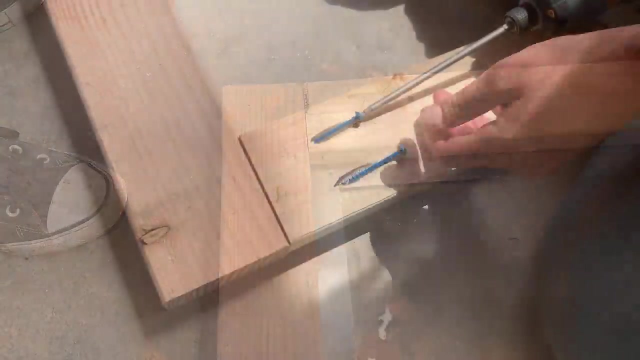 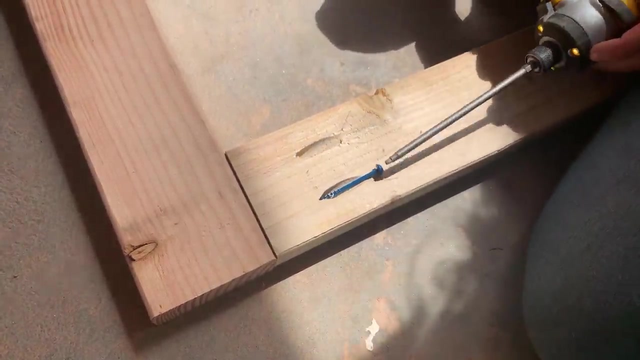 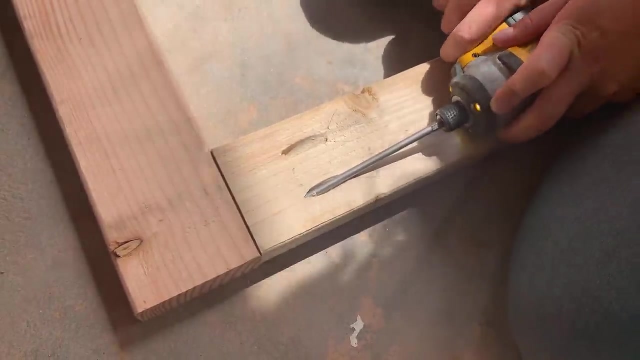 These are the blue screws that I was talking about. These are all weather screws Made for outdoor usage And they make them different lengths. Of course, they make them to use in 2x material, The easiest way to cut out the piece for the center. 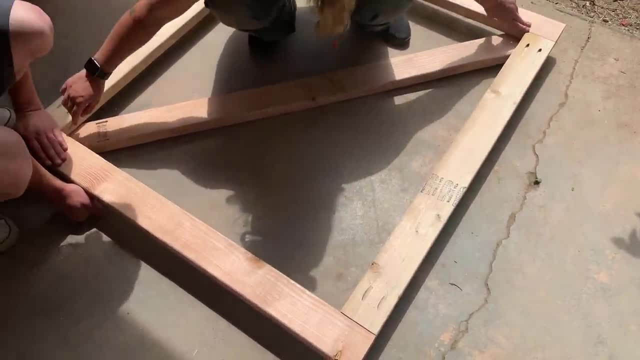 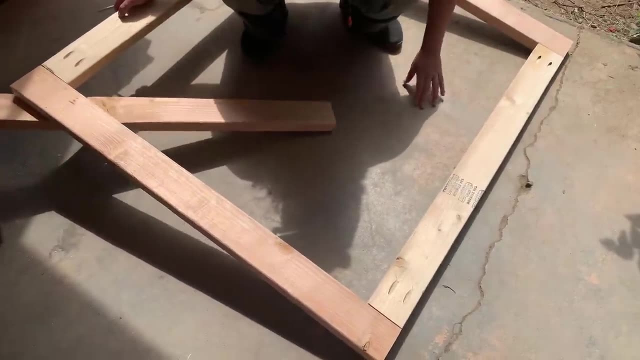 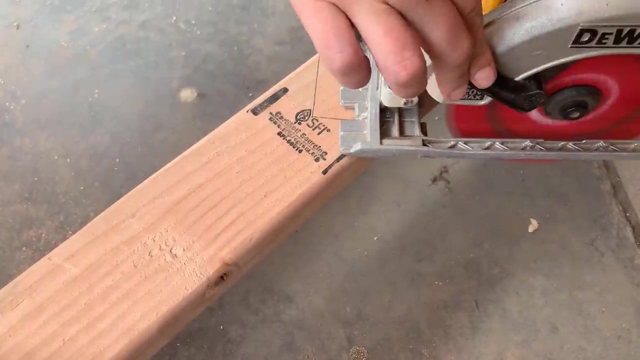 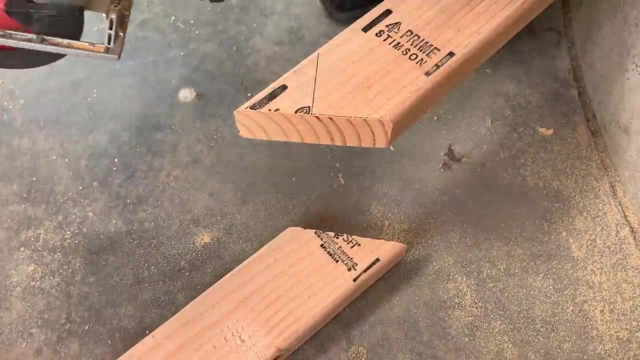 Is simply to set the square gate on top of it And then trace out Where you want to cut this diagonal brace, and of course that's easy enough to cut with a circular saw. I got a few comments about Maya's use of the circular saw when we did our shed build and how. 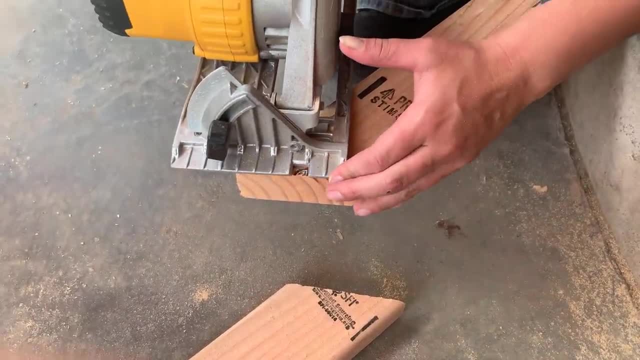 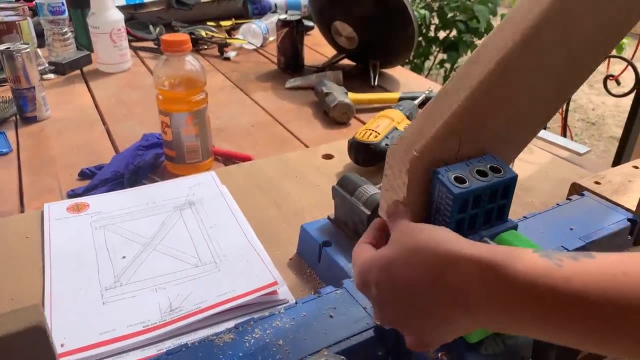 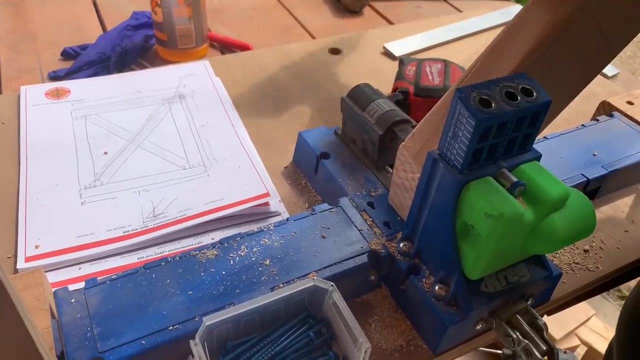 people might be concerned with her hand placement and that she might not know where the blades at, but I just want to assure everybody that she's probably cut thousands and thousands of boards in the last 11 years or so that she's been using a circular saw and she knows exactly where the blade is at all times. 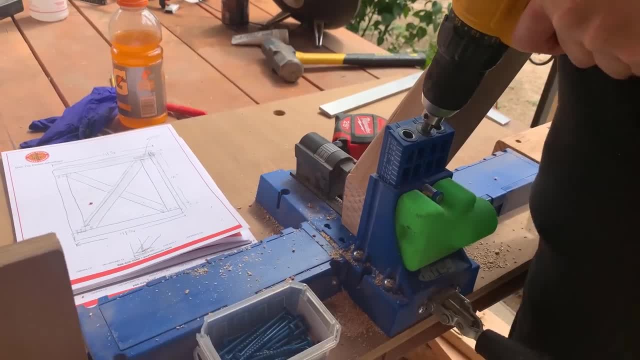 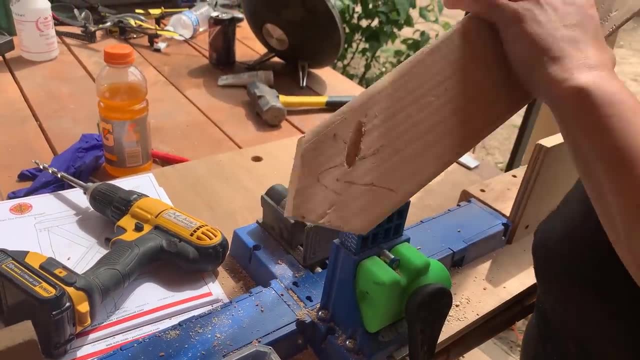 And of course we're just going to use pocket screws for this assembly as well. We'll put one pocket screw in each of the the two faces there, so one will go into the side rail of the fence and one will go into the bottom rail or top rail. 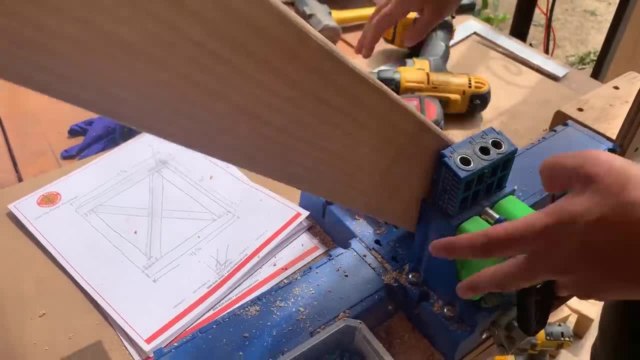 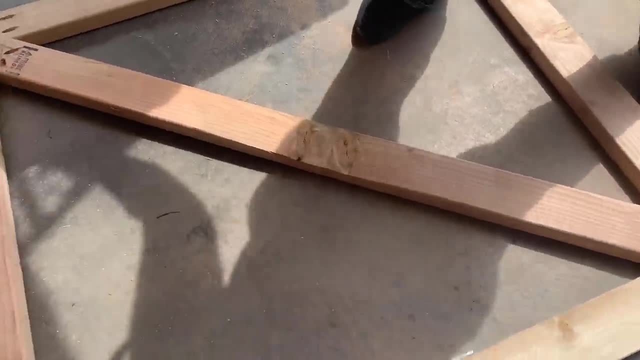 as it were, and that'll lock this diagonal brace in. So we're just going to put one pocket screw in each of the two faces there. so one will go into the bottom rail, or top rail, as it were, and one will go into the bottom rail, or top rail, as it were, and one will go into the bottom rail or top rail, as it were, and that'll lock this diagonal brace in. 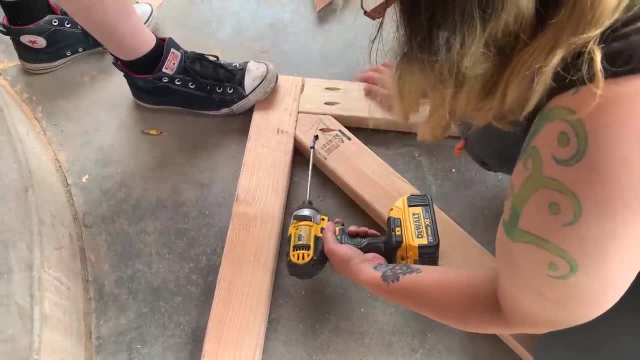 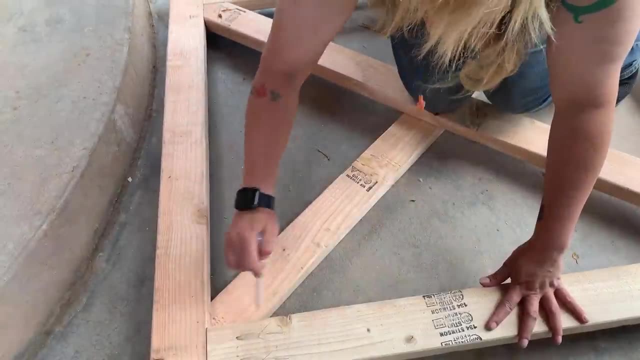 Once you get these diagonals in, it really locks up the strength of this gate and the gate isn't going to sag over time and this also helped just to keep it rigid. We're going to do another brace in the middle and we're going to 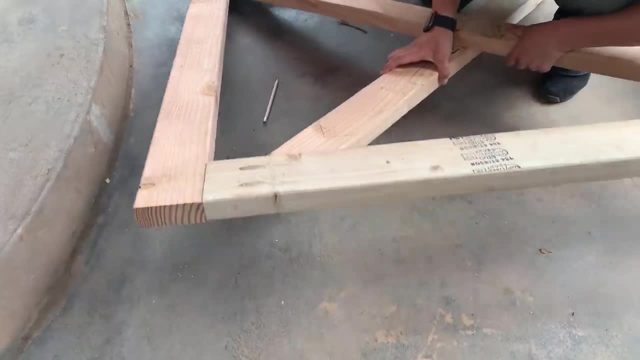 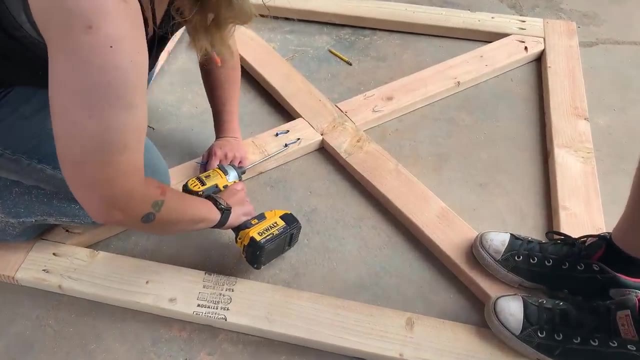 do the same thing. We'll set the brace underneath the gate itself and we'll draw lines where we want to cut it off and we're also going to pocket screw that and we'll put that together in the exact same way. And this is a. 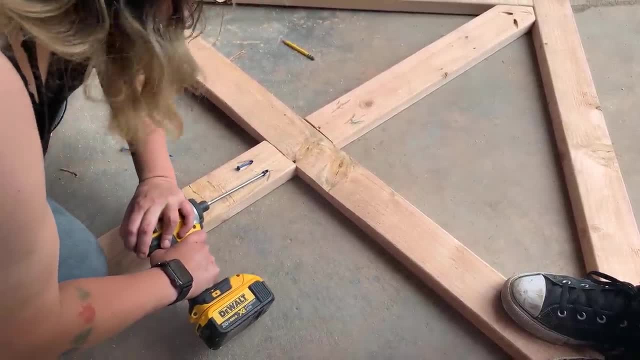 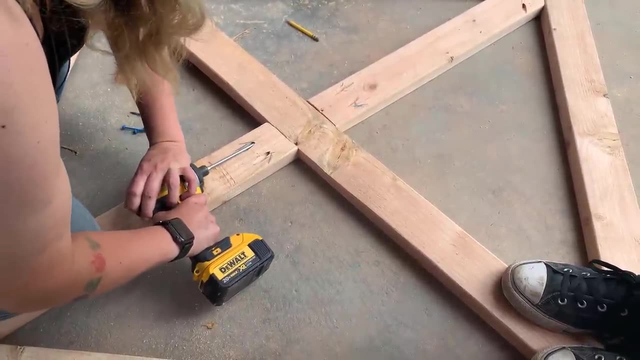 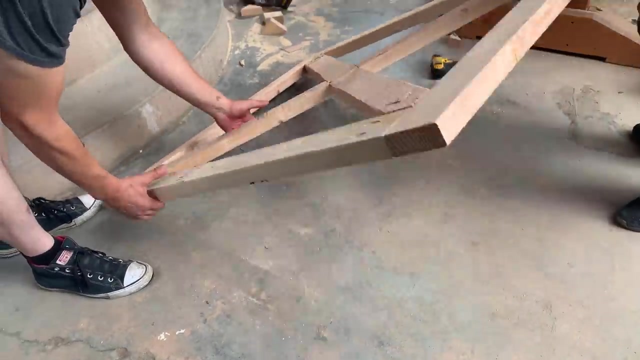 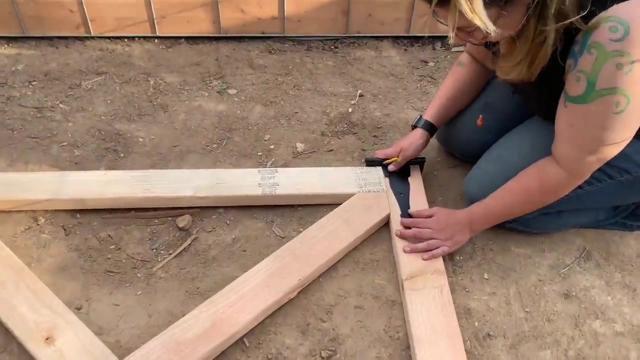 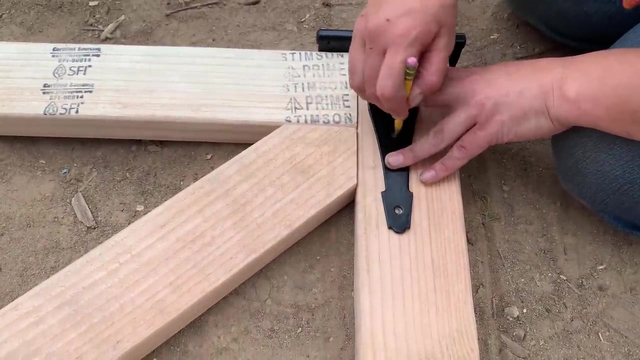 little X-frame that I was talking about and that really will complete the structure of the gate. Next, we're just going to put normal fence-mounting hardware on it in order to attach it to the planter garden itself. Once again, I just want to give a shout-out to my viewer and friend, Eddie Cortez. 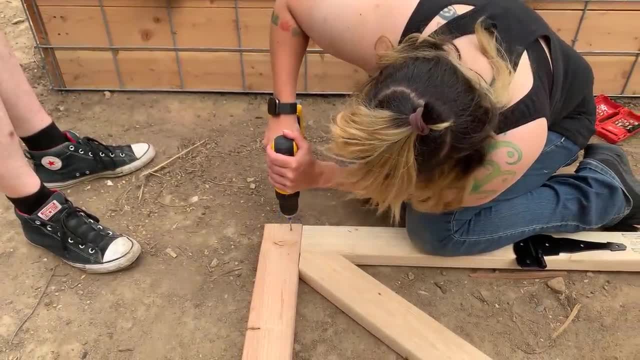 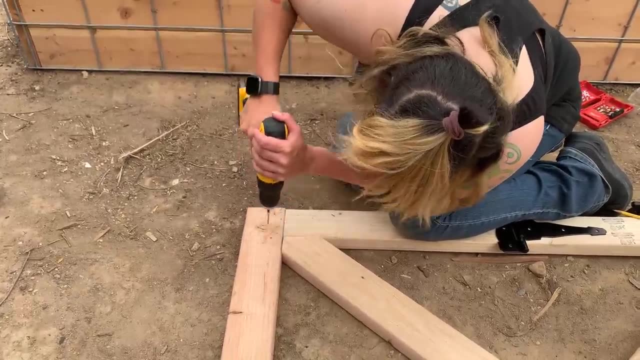 who sponsored this build And if you guys found this build interesting at all, if you enjoyed it, you might want to check out their website- Him and his wife. they have a website. It's called bathhandmadecom. It's B-A-T-H-E handmadecom. 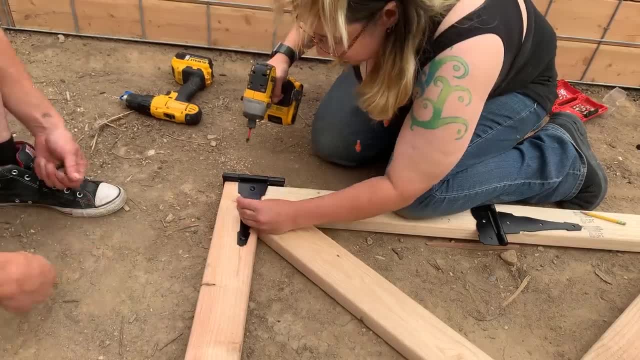 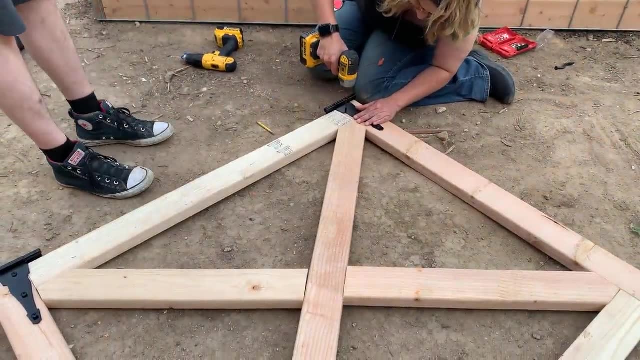 And they sell bath products, I think, candles, soaps, things like that. It's a great website. They're really good people. So if you're in the market for something like that and you like this video, then maybe check them out and see if there's something there that you need. 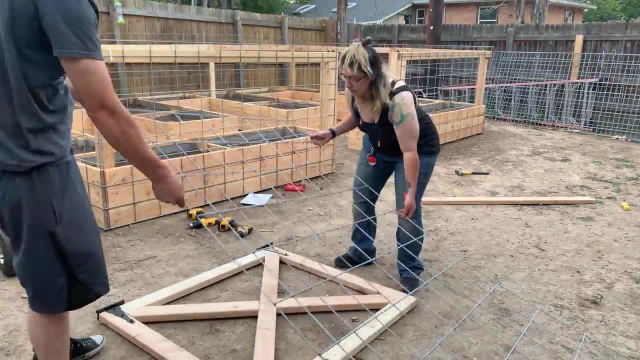 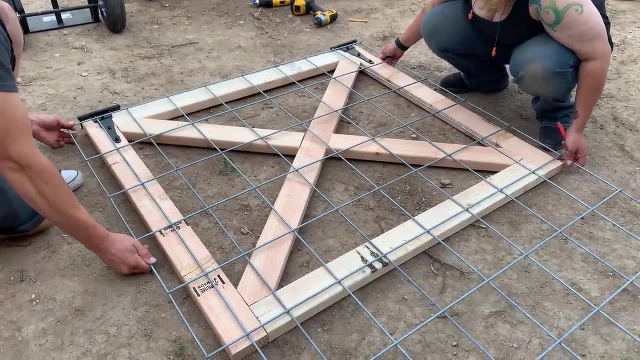 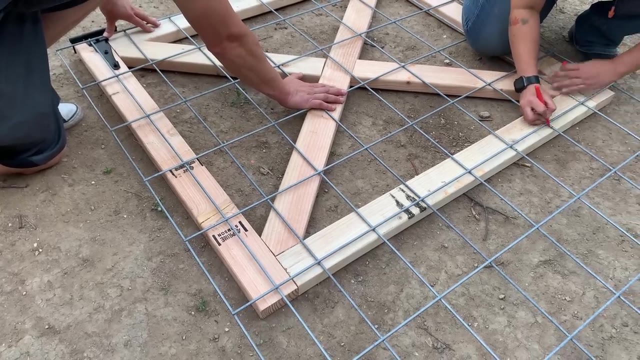 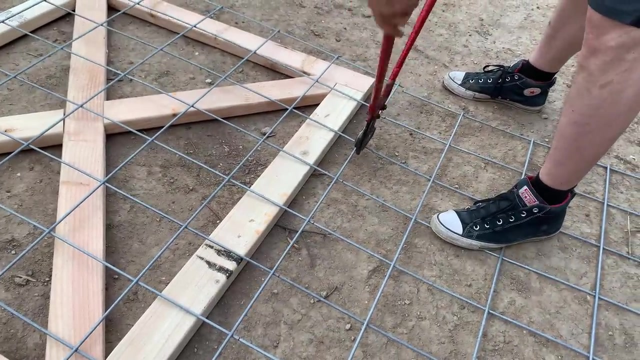 I'll put a link to their website in the description down below. And thanks again, Eddie. So if you end up doing something like this and you get any of this cattle panel to work with, you'll find that these bolt cutters really make it easy to cut. 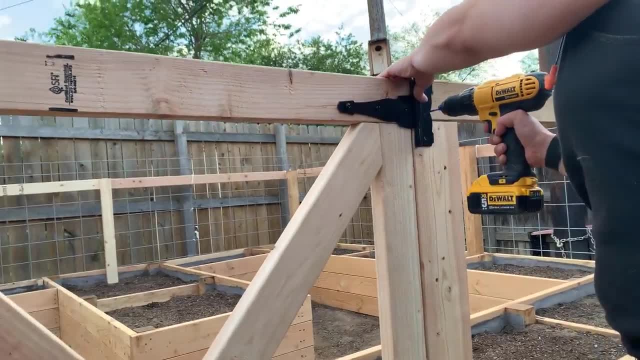 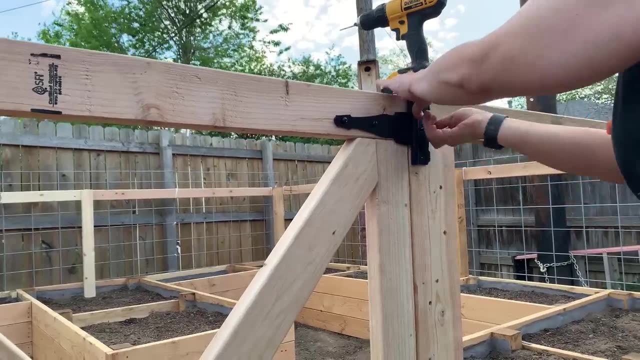 You could easily cut it with a grinder or a hacksaw, but it's going to take forever. compared to the speed of the bolt cutters, We found it was easier to put the gate up before putting the wire on. This allowed it to go on a little bit easier without the wire in the way. 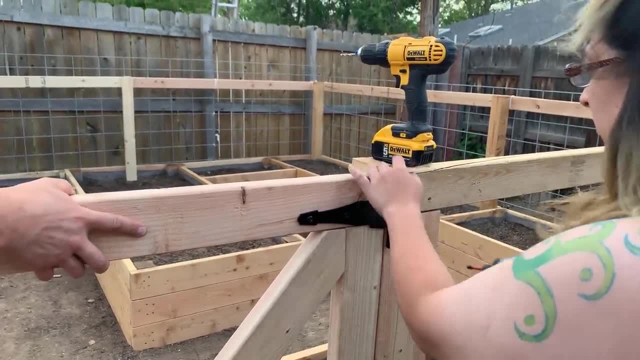 We're not carrying the weight of the wire with it. And then, of course, on the wall side to the right, there we can just put the wire right over the hinge, And I think that that's going to make it a lot easier. 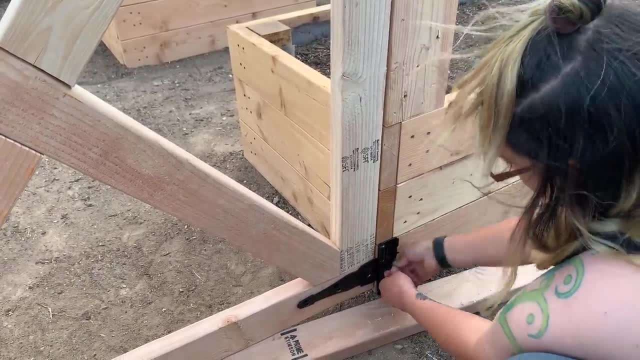 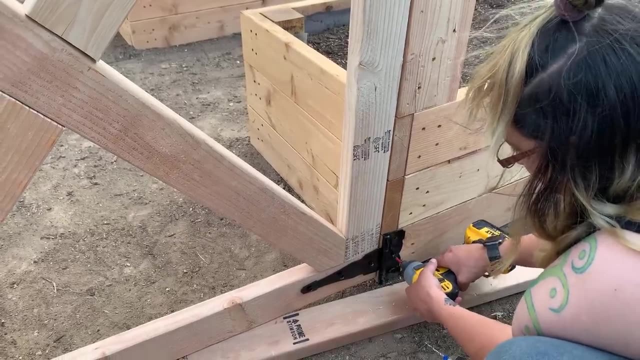 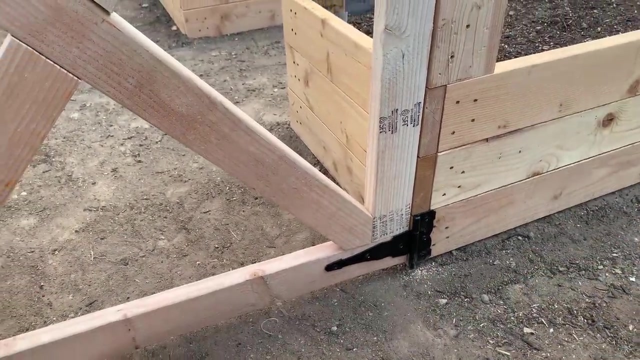 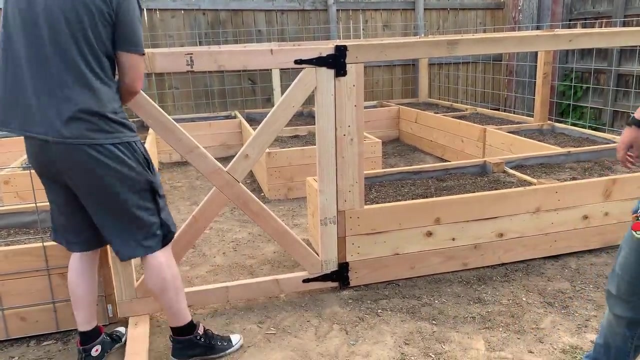 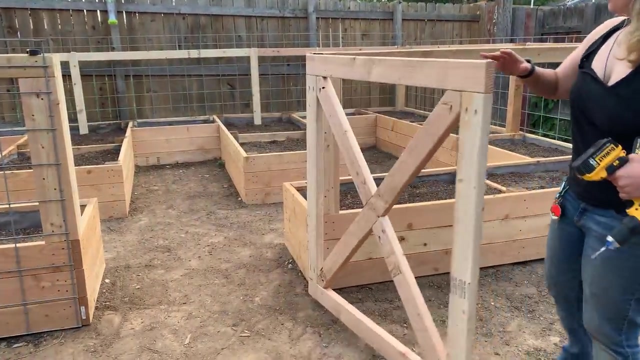 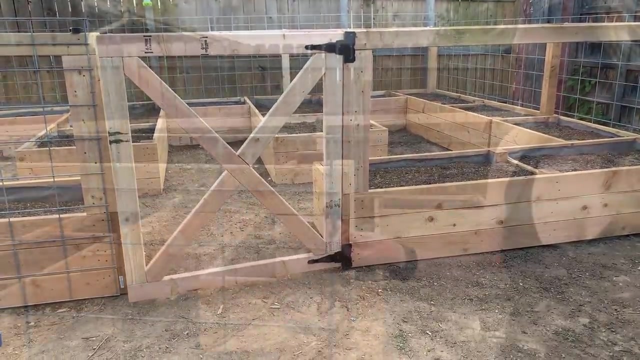 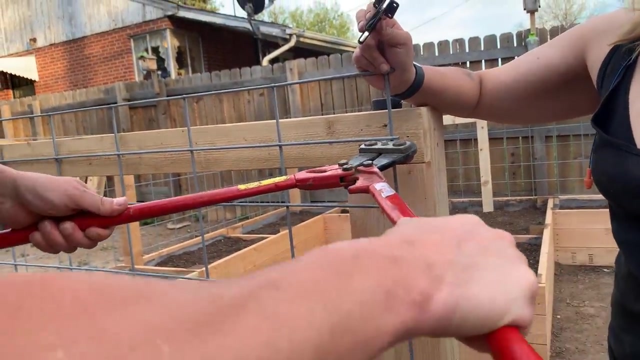 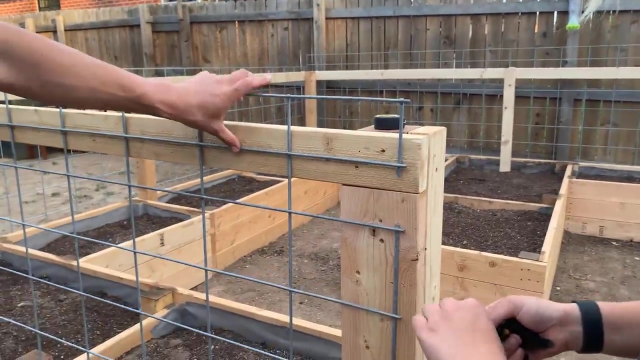 Subtitles by the Amaraorg community. And of course we're going to need a latch, otherwise Lily is going to find a way to open that gate and get in there. So we didn't secure this corner of the cattle panel down because we knew we'd have to trim. 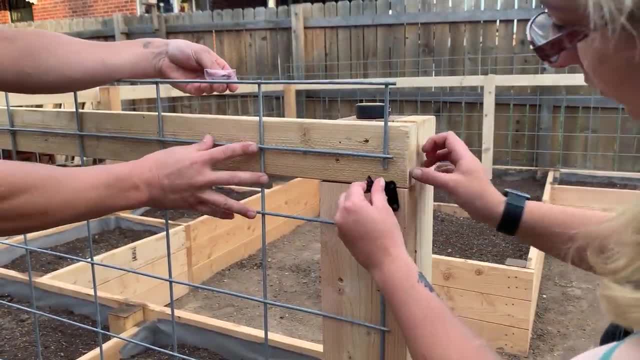 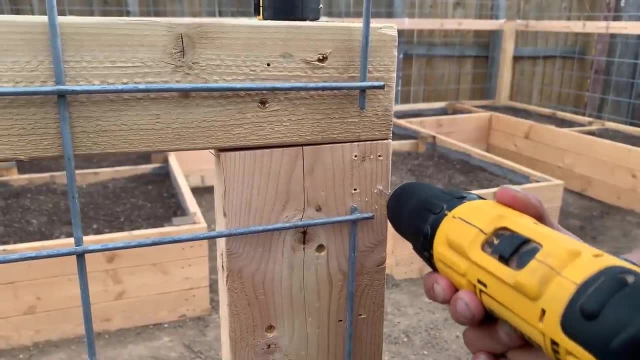 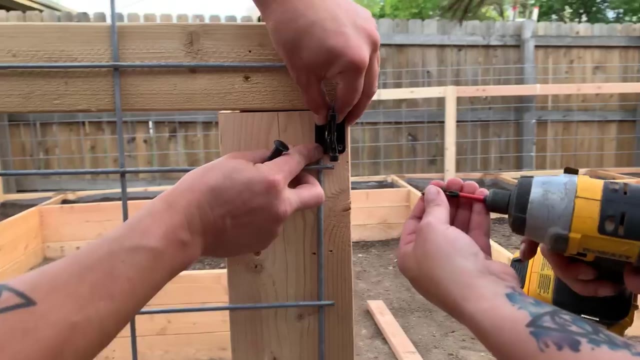 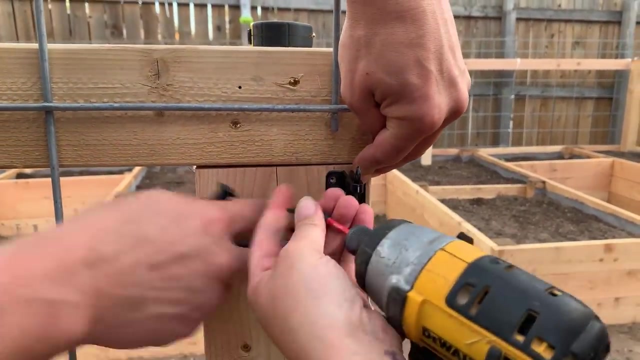 out a little section of it in order to get the latch on, And so Maya's boyfriend has done that, and so they're going to go ahead and attach that latch next. A lot of this stuff, you don't necessarily have to pre-drill. 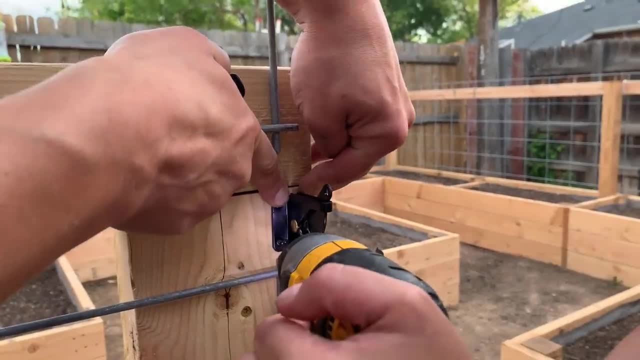 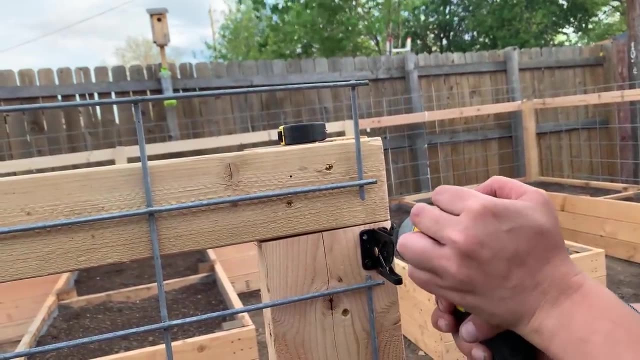 I tend to pre-drill gate hardware. However, I'm putting it in because it's usually in the spot that I definitely want it to go and I don't want to end up splitting a board and, you know, maybe having to relocate a latch. 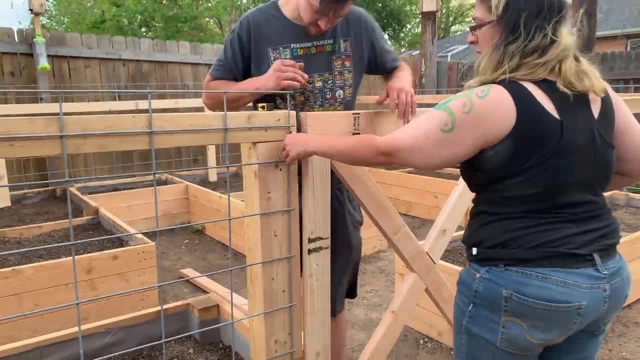 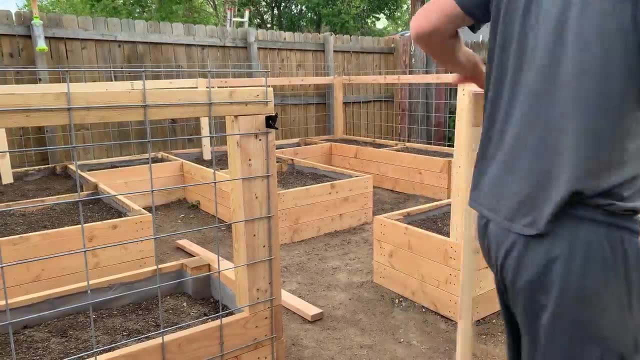 or relocate a hinge or something like that. So when it comes to stuff that I want to make sure, you know if I've only got one place to put it, then I usually always will pre-drill, And it looks like the gate functions pretty well there. 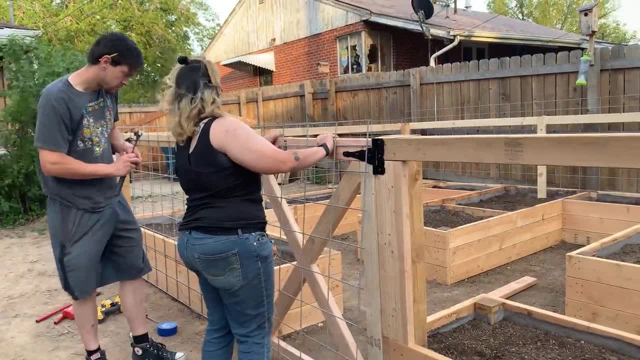 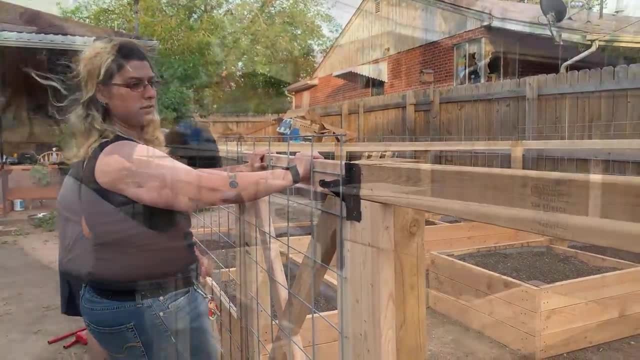 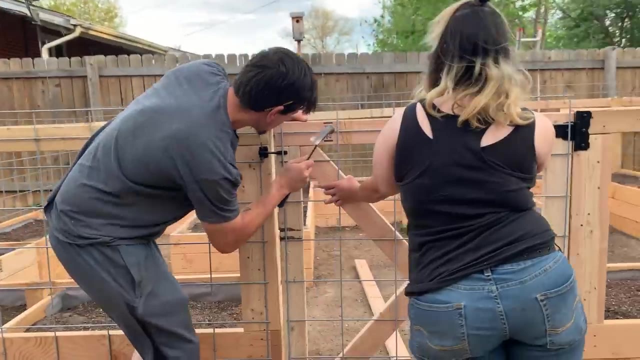 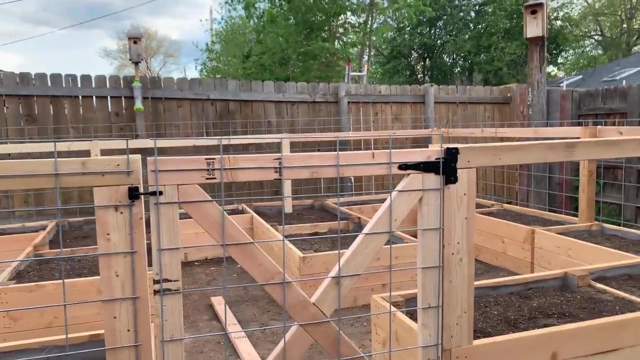 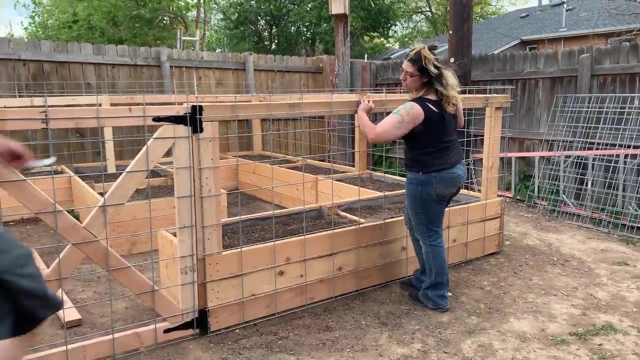 I think the next step is to get some metal on it. Okay, Okay, Let's take a look. Okay, Once again, if you guys want to build something just like this, I will have a link to the plans in the description down below. 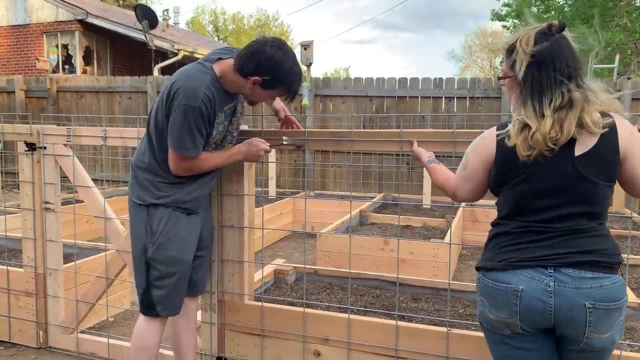 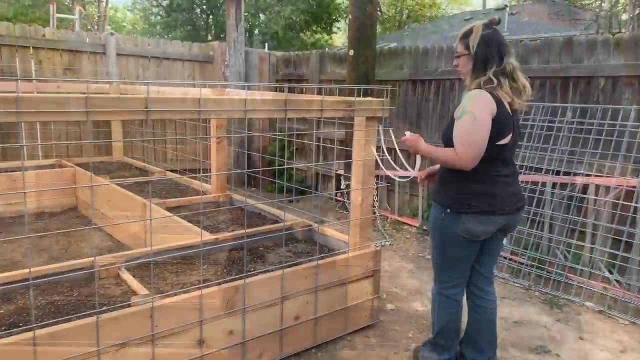 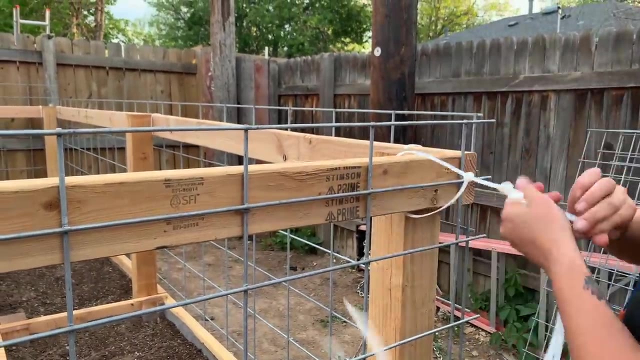 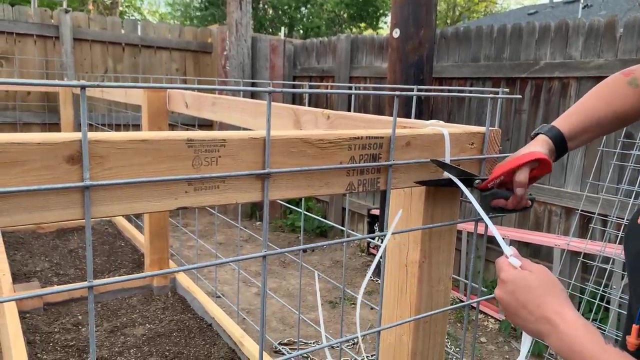 Okay, Okay, Okay, Okay. and here's around the corners. I said we'll put some zip ties. these are pretty heavy-duty zip ties- I think they're 24- and zip ties they're ready to hold 175 pounds. so we put a few of these around the corners just to give it a little bit. 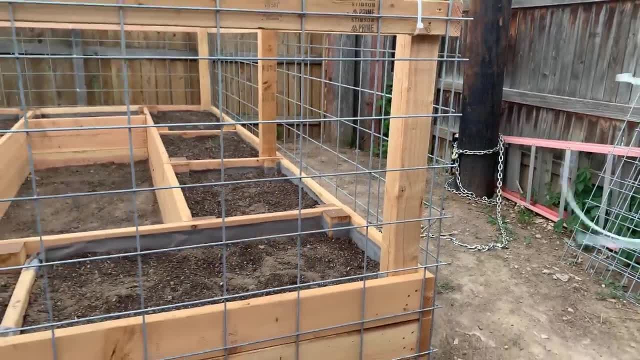 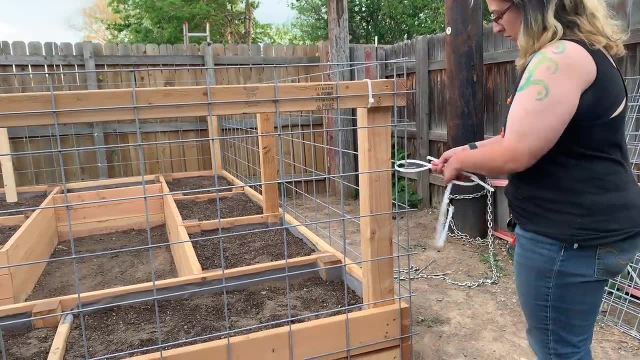 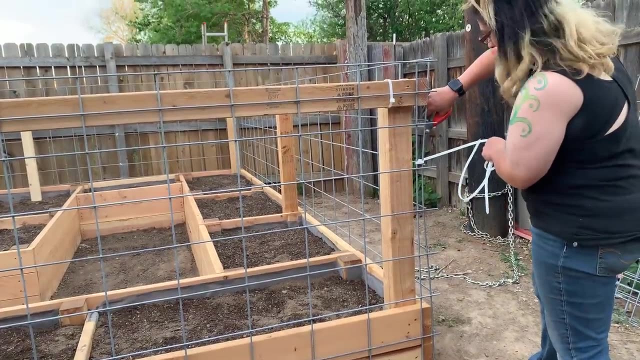 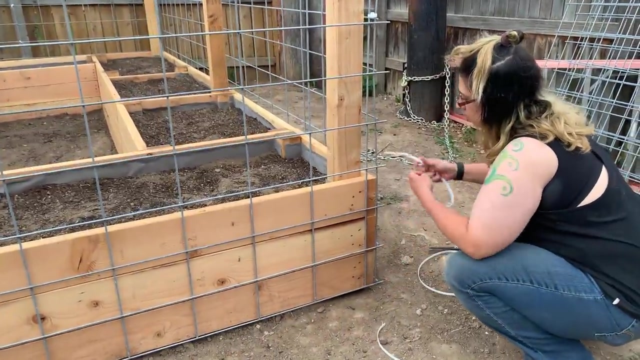 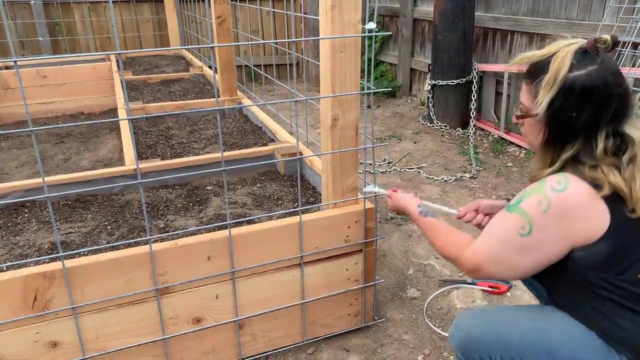 of extra strength until we get the u-bolts in. not a hundred percent, sure if these are necessary, but we decided to put them anyhow. we got these things on Amazon. I think it was around $15 for a pack of 50 of them and they're pretty handy. we actually used them to put some pretty cool stuff. 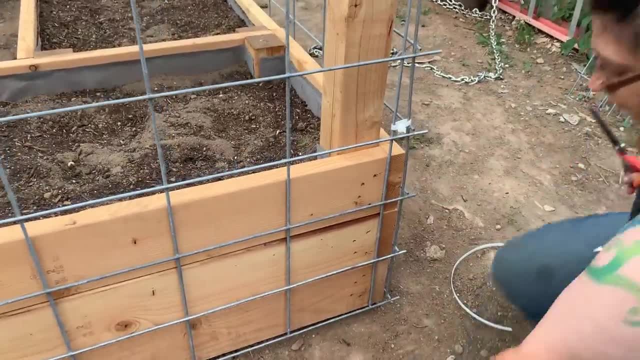 up some archways and stuff like that, and then we're going to go ahead and put these things on Amazon. I think it was around $15 for a pack of 50 of them- inside of the garden area too afterwards. so you'll kind of see some glimpses of 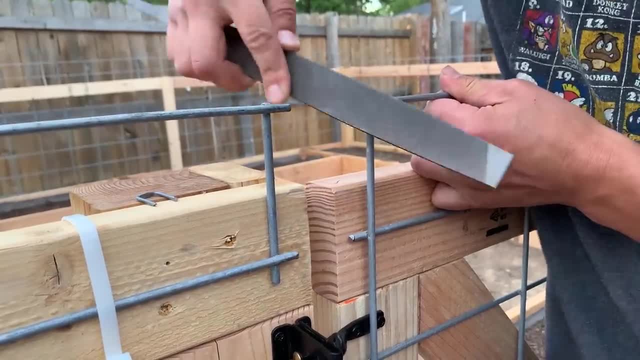 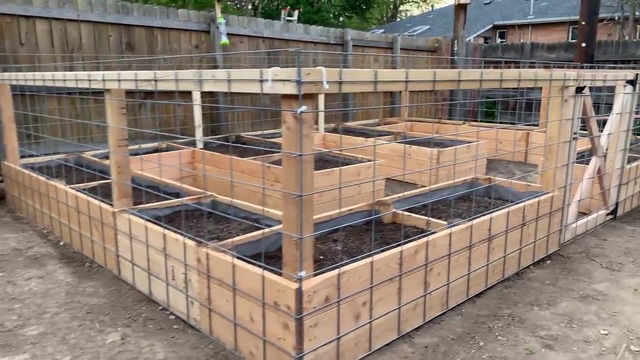 that right at the end. then we did go back through and just kind of hand file the really sharp edges of that wire where we cut it on the way in and out of the gate so we didn't get poked on it. and there you go. this is kind of the 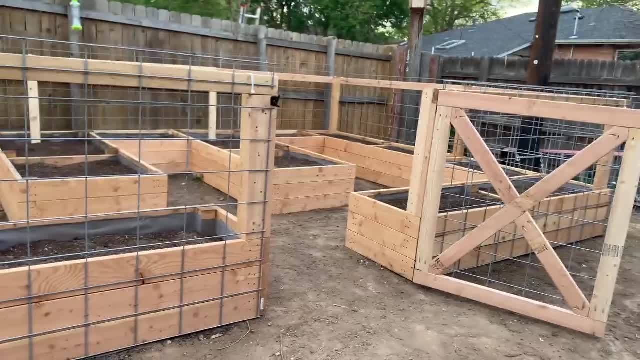 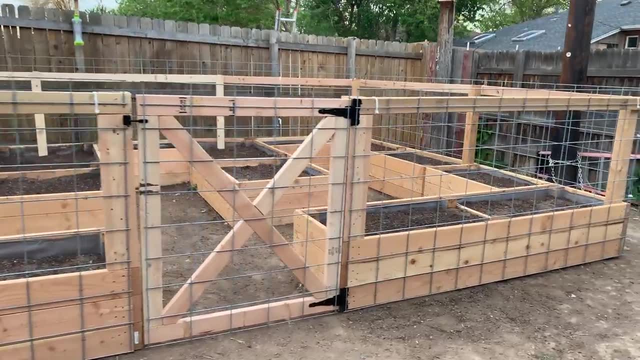 preview of what this looks like. you can see it's got distinct walkways in there and all the walkways are three feet wide and every area that has planting can be easily accessed from the walkway. the planter boxes which are in the very middle are a little bit wider than the 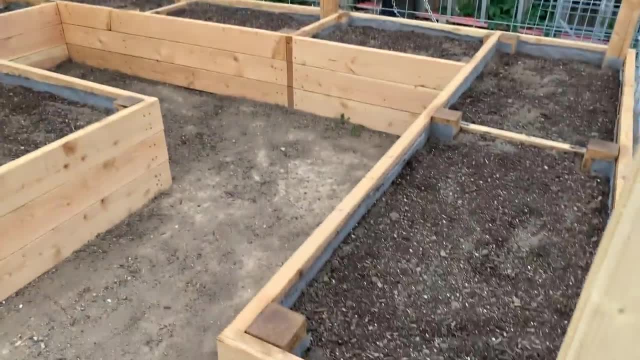 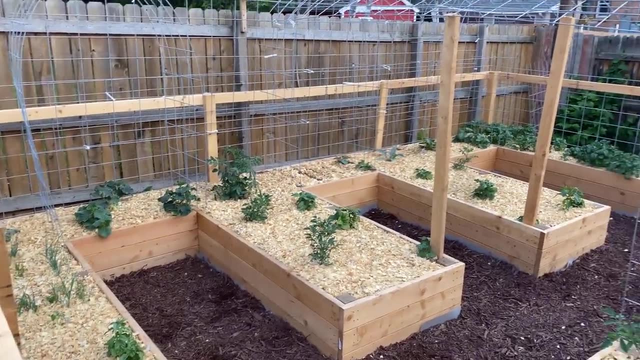 planter boxes around the perimeter because those can be accessed from either side. I hope you guys liked this video and if you did, it would really appreciate it. if you could click that subscribe button down below and if you click the little bell icon, that will notify you of future videos that we have. 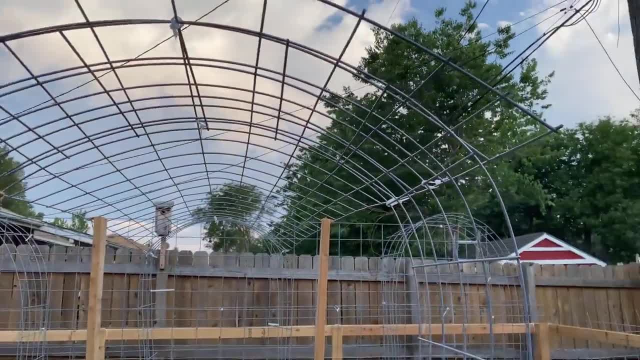 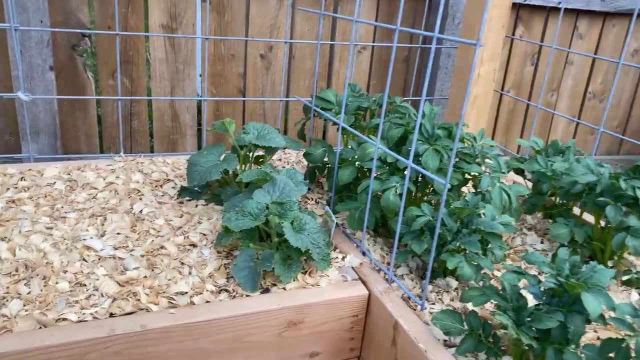 coming out and I'd like to say thank you to all my patreon supporters and if any of you are interested in helping to support the channel, we do have patreon, and there's a link to that in the description below too. that wraps up the build for today. I'm going to end with a couple of more shots.